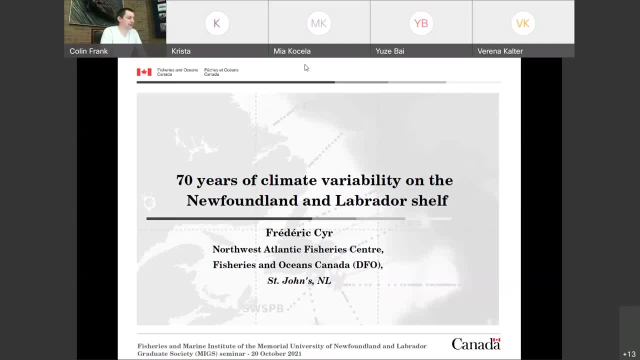 and the relationships between biological, chemical and physical properties. So now, Dr Cyr, I'll let you begin with your presentation. Oops, All right, thank you, Colin, and thank you everyone for being here. Thanks for the invitation. That's pretty cool to be in person, finally, after a little while. 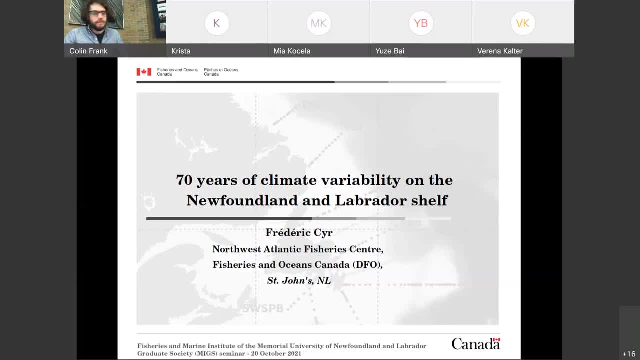 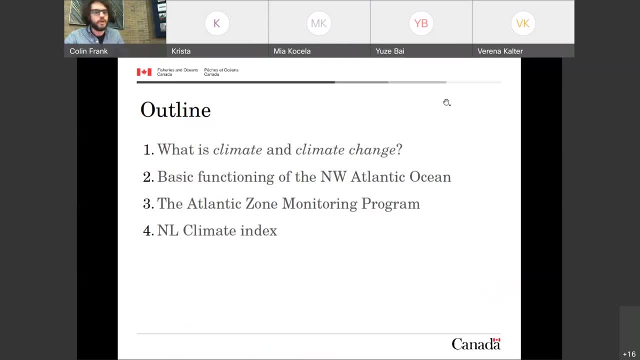 So my talk will be about the ocean climate in Newfoundland and Labrador. All right, so here's my outline. Very broadly, I'll define what is climate, what is climate change, Then I'll give some basic functioning about the Northwest Atlantic Ocean. 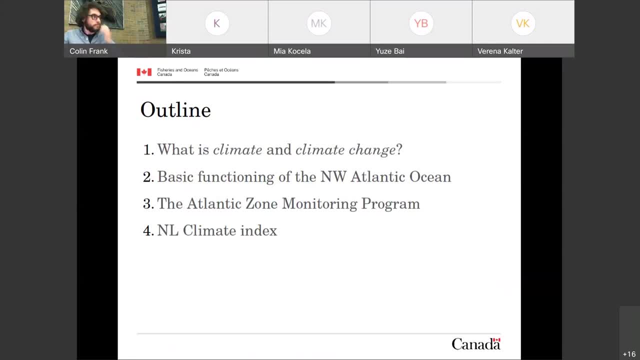 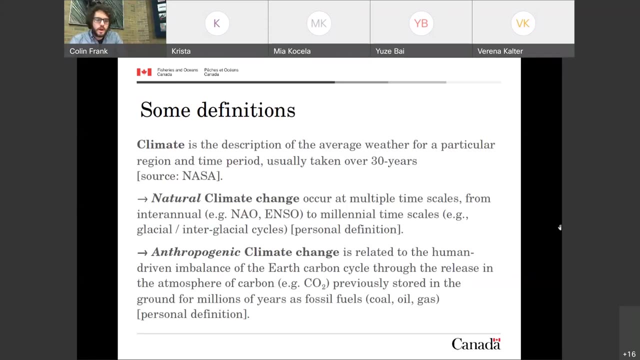 Then I will talk about the Atlantic Zone Monitoring Program, which is basically the core of my work, And then I will introduce a new index that was developed recently for climate studies and ecosystem studies. So first some definitions. So climate is the description of the average weather for a particular region and time period. 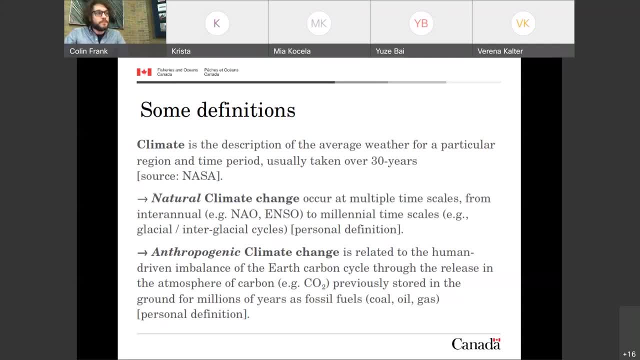 usually taken over 30 years. The reason why we generally 30 years is a standard from the World Meteorological Organization. The reason we use 30 years is only because it's a handy timescale for humans, something we can refer to when we talk about the changes in the weather. 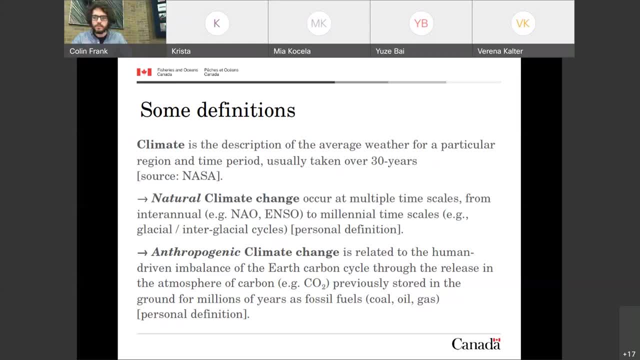 Then I would like to differentiate the natural climate change which occur on multiple timescales from inter-annual, for example, driven by phenomena like climate change Phenomenons such as the North Atlantic Oscillation, NAO or the El Niño Southern Oscillation. 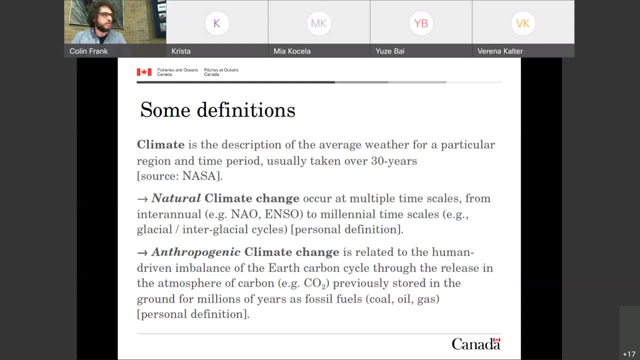 to something much longer, to millennial timescale, for example, glacial or interglacial periods. So this is a natural climate change. What we hear in the news. when we talk about climate emergency, we refer to the anthropogenic climate change which is related to the human-driven imbalance of the Earth-Carbon cycle. 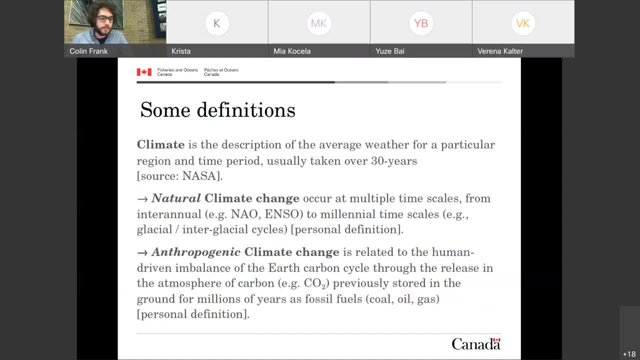 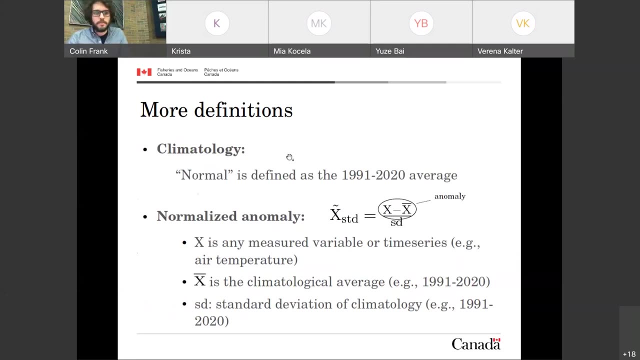 With a release in the atmosphere of carbon, for example CO2,. it was previously stored in the ground for millions of years under the form of fossil fuels. Going a bit further into definitions and kind of piggybacking on this, I would like to define what is a climatology. 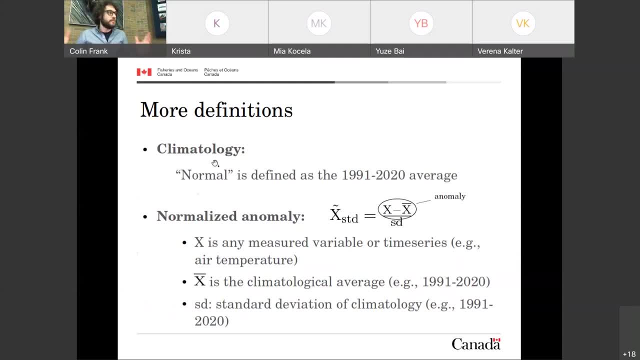 So a climatology, or what we consider the normal or expected weather, is defined as the average over a 30-year period, the famous 30 years that I mentioned before. Again, this is a WMO- World Meteorological Organization- standard. 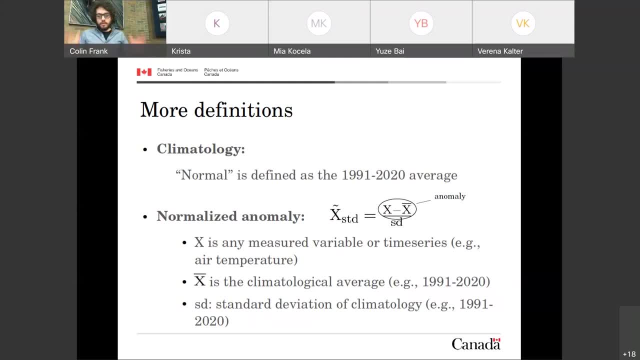 Every 10 years we shift our reference period by 10 years. Every 10 years we shift it, So since 2020, we're into 1991, 2020 average as the normal. So using climatology we can define what is a normalized anomaly. 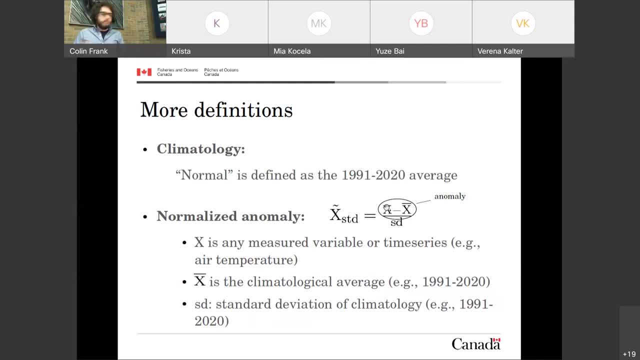 So let X here be any measured variables: temperature, salinity, sea ice, wind speed, whatever. So if I subtract from X, a certain year, the average of that variable over the climatological period, then I get what I call the anomaly. 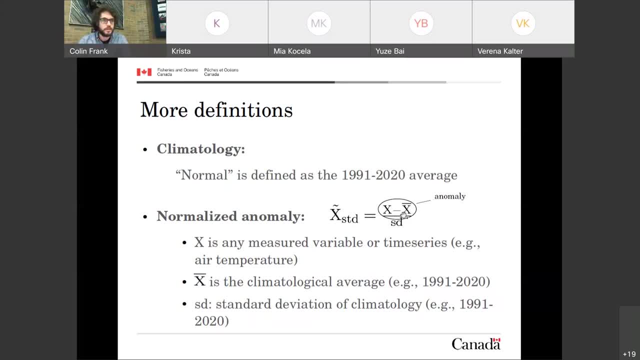 So that would inform me. for example, last year was 1 degree Celsius above average. If I divide this anomaly by the standard deviation of again that variable over the climatological period, then I get a unit-less quantity. It's called normalized anomaly or also standardized anomaly. It's handy because it's unit-less. You can compare different quantities together. You can compare temperature, salinity, wind speed, et cetera, all over the same scale. In this sense, the scale would be: last year was 1 standard deviation above or below average, for example? 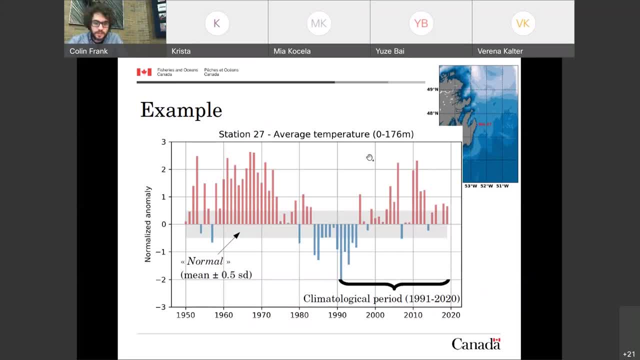 Just a quick example of what it looks like and to illustrate that this is data from Station 27,, which is one of the longest high-speed railways in the world. This is a data from Station 27,, which is one of the longest high-speed railways in the world. 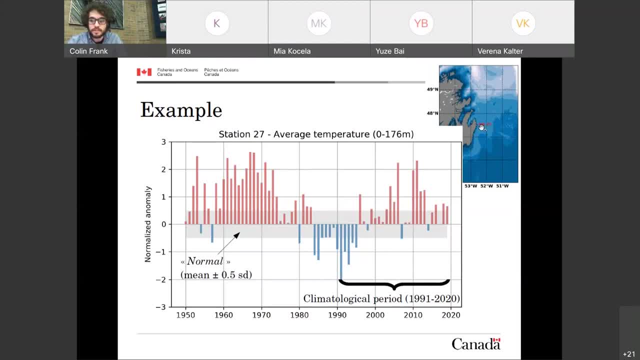 This is a data from Station 27,, which is one of the longest high-speed railways in the world. This is a reference to Geographic Times here in Canada, located here just outside St John's Harbor. This is a reference to Geographic Times here in Canada, located here just outside St John's Harbor. 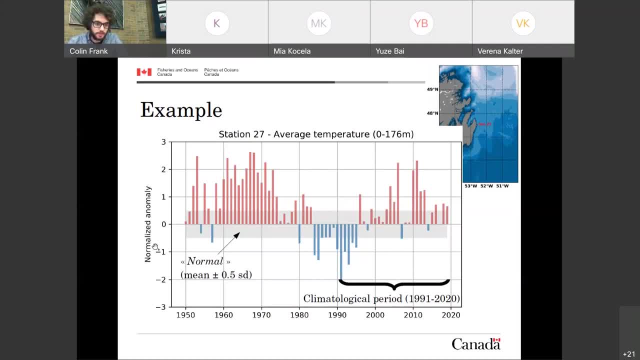 What you have here is the normalized anomaly in terms of standard deviation since 1950, of the average temperature top to bottom, January to December. What we see is that, for example, in the 60s we were 2.5 standard deviation above a longterm average. 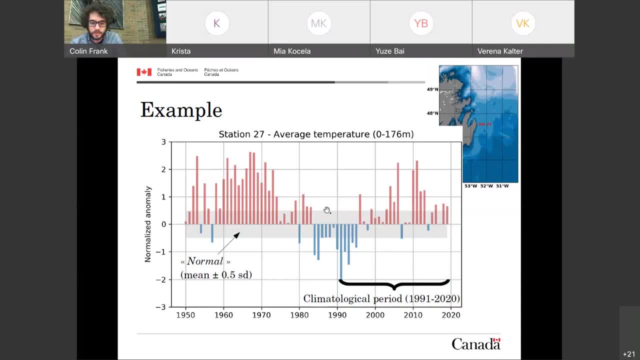 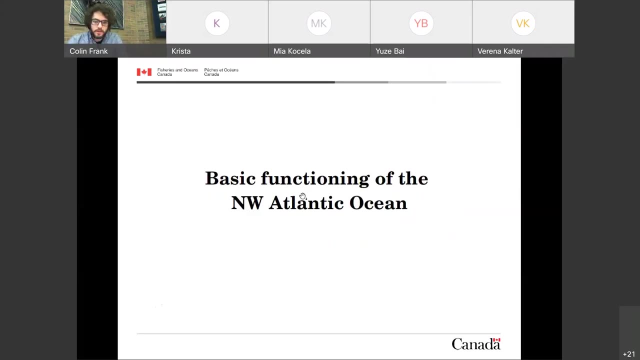 which is based on this period here: 1991, 2020.. So everything is scaled towards this period, and then we can see the cycles in the climate. So this will come back throughout my presentation, so I thought I would introduce that from a start. Now let's talk about the 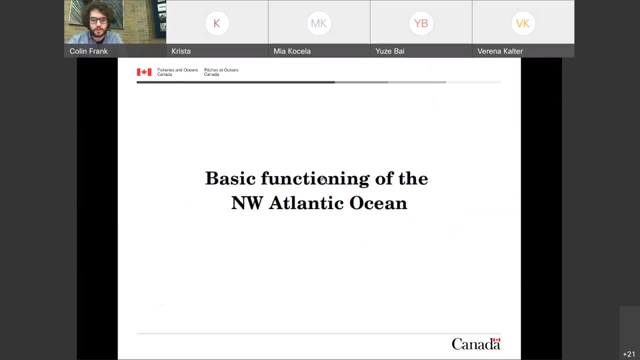 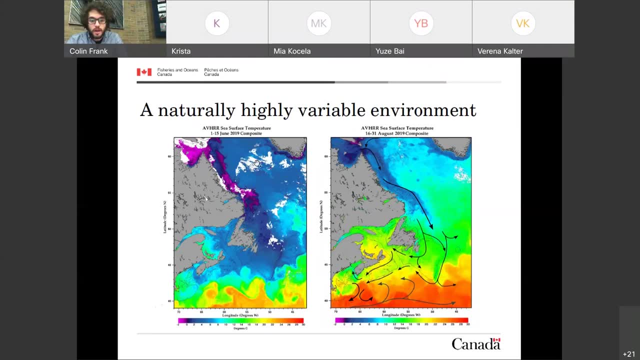 Kind of a basic functioning of the Northwest Atlantic Ocean. So the Northwest Atlantic Ocean and especially the Newfoundland Labrador Shelf Are a naturally highly variable environment And to illustrate that I show you here to see surface temperature composite from satellites. The 1st 1 here is from the 2 1st week. 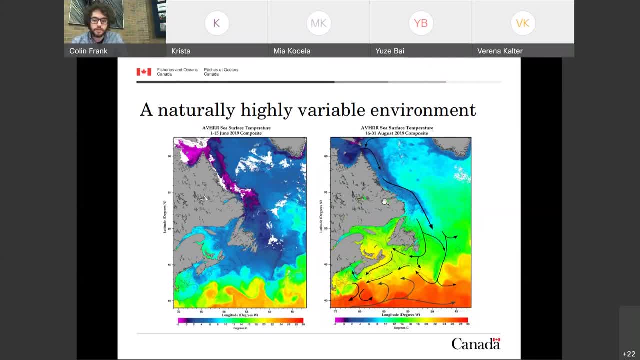 Of June 2019, and the 2nd 1, the 2 last week of August 2019.. So late August is basically the warmest time of the year, And even in the warmest time of the year, we still have close to 0 degree Celsius water flowing on the shelf here. If you look at a color scale, dark blue is 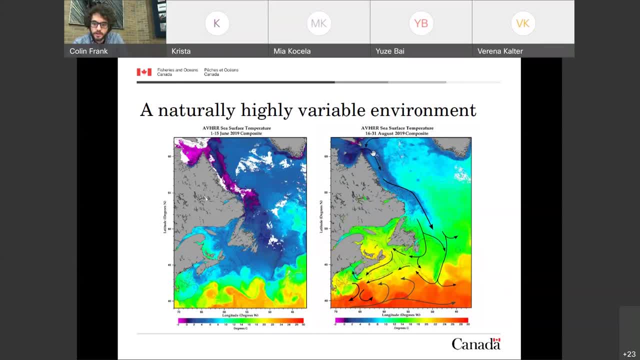 Close to 0, and purple here is sub 0. So even in the warmest week of the year we have this Very cold flow on the Labrador Shelf, Meeting at some point the warm water of the Gulf Stream here close to 30 degrees Celsius. 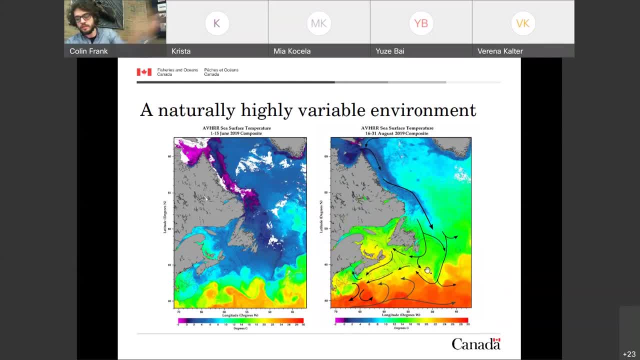 So in few hundreds of kilometers we go from nearly 0 degrees Celsius to 30 degrees Celsius water, Just in the region of the of the Grand Banks and And St Joe's. so This region is naturally highly variable, just because of this fine balance between the cold water coming from the north. 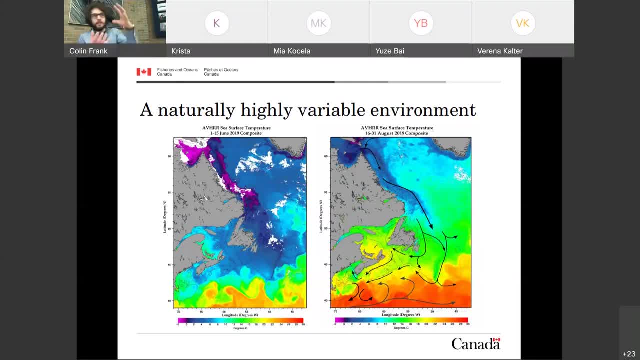 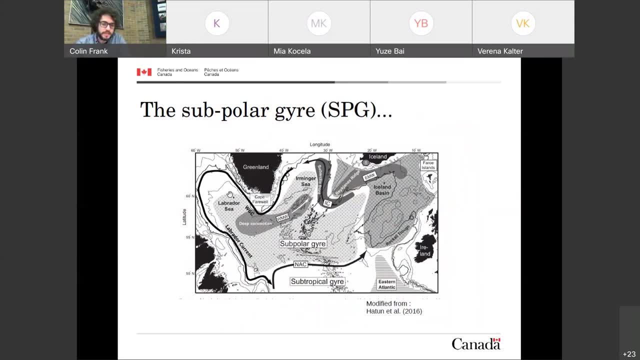 And warm water coming from the south. so any change in the positioning of this current would change the ocean climate a lot. And to understand this again, find balance between the different current, We need to understand the sub polar gyre. So the sub polar gyre. 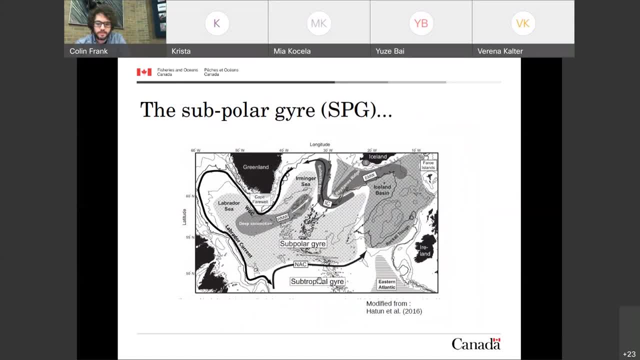 Is kind of this: sets of currents: here There's a Labrador, There's a Labrador current here on the flowing, on the, On the shelf edge. here then the North Atlantic current, which is the Eastward extension of the Gulf Stream, bringing 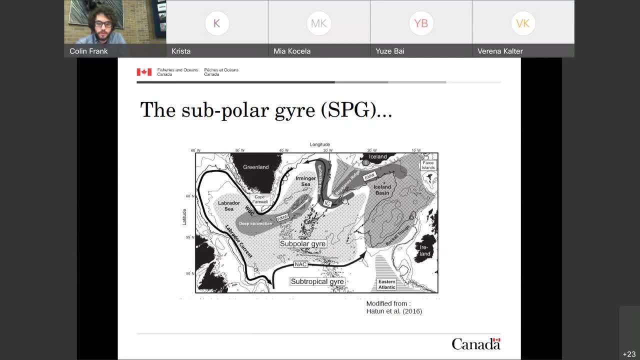 Warm water towards Europe and then there's a loop back with the earning, your current, the East and West, green and current, So it is kind of average Pattern of the current. of course the water properties are changing from As as the move, for as they complete the loop. 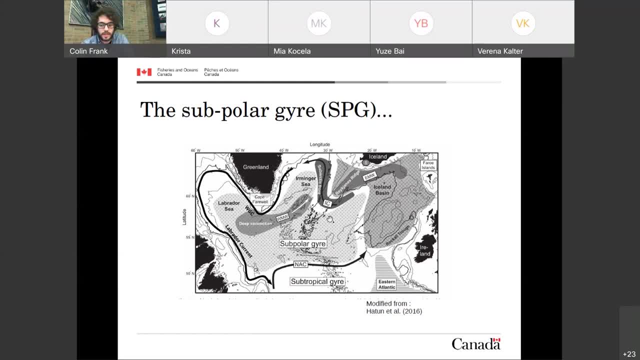 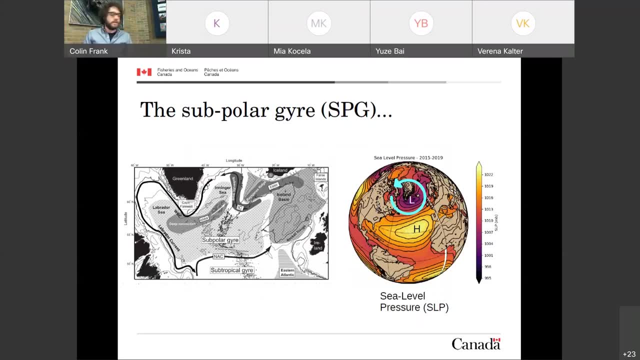 But it's basically what is the? the average current in the North Atlantic And the sub polar gyre is set in motion By the mean winds above Above the Atlantic and the mean winds are are Are set in motion by the difference in sea level pressure. 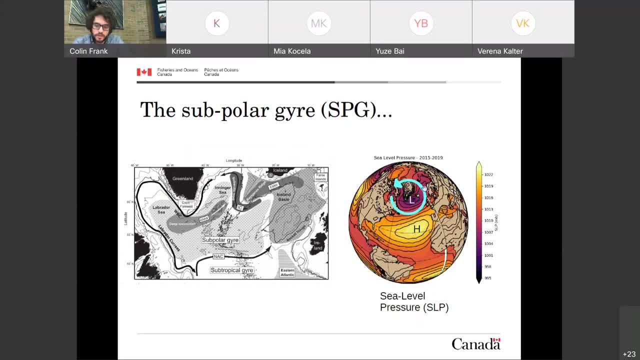 Above the North Atlantic. and I try to kind of Do a sketch of the mean wind pattern here with this arrow, Because in geophysical fluid dynamics The flow is perpendicular to a pressure gradient. So this in color here what you have is the um. 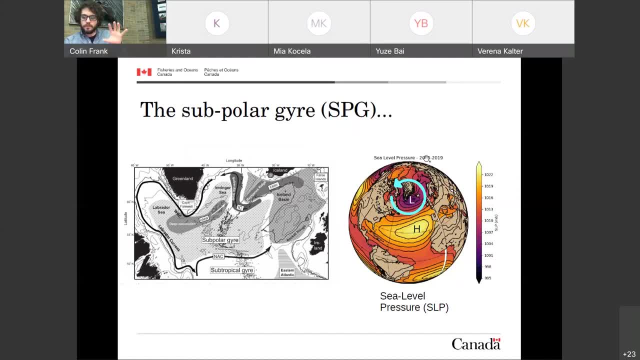 Sea level pressure. uh, For this 5 years average, 2015,, 2019.. So there's a high pressure here- look at it near the- and a low pressure near Iceland In this pressure gradient here will drive a Flow perpendicular to it because of the rotation of the earth. 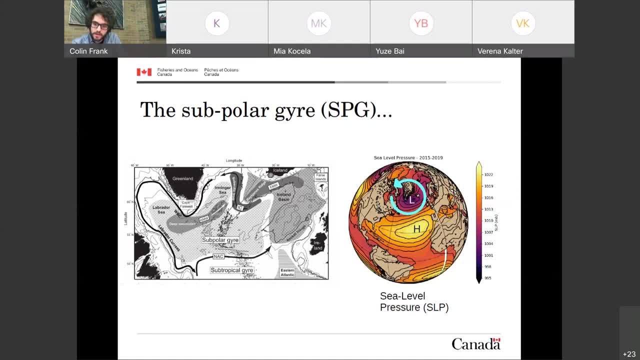 So this is what we call here the Western release, And there's a return flow from the Arctic bringing cold air towards our region. So this is basically The this um sea level pressure pattern drives the air flow, which in turn sets the sub polar gyre in motion. 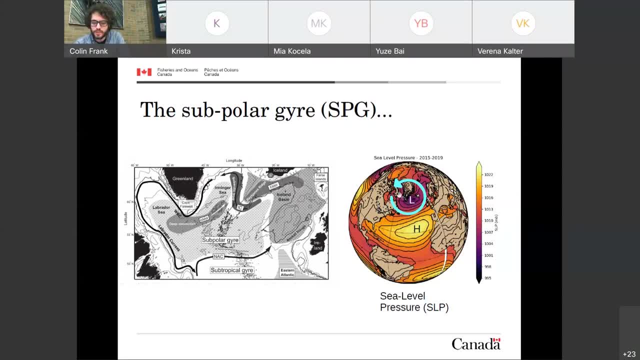 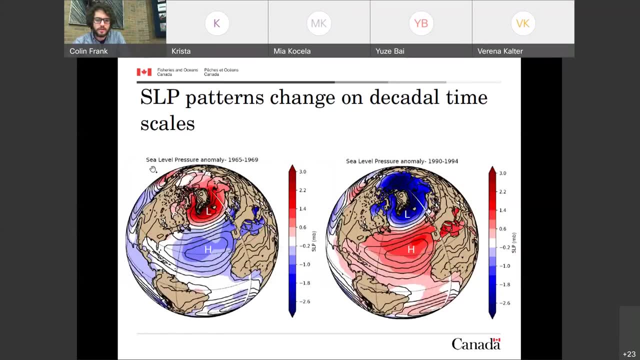 The thing is that these uh sea level pressure Changes from 1 decade to the other. Um and the next slide I show the sea level pressure anomaly. So the difference between These 5 year period- the 1st period is 1965.. 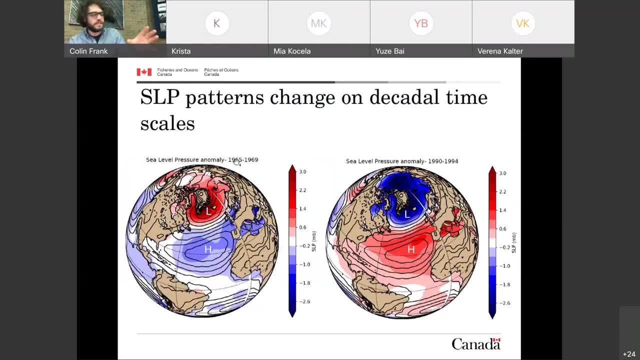 Well, basically the sixties and the nineties, so the 1st. in the sixties The low pressure here was a few minute bar higher than usual And the high pressure here was a few minute bar lower than usual. Well, in the nineties the low pressure was lowered. 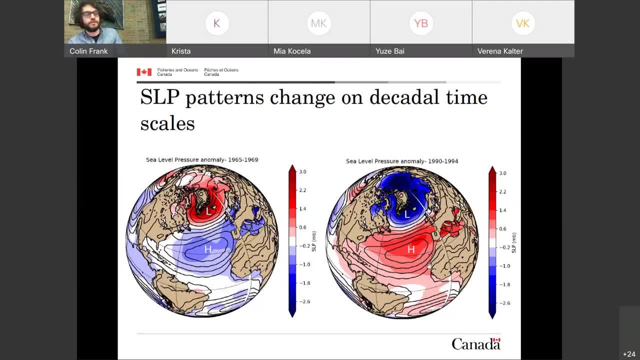 High pressure was Higher, meaning that the difference here is greater. So there's a stronger airflow in the nineties compared to the sixties, for example. This leads to colder weather in Newfoundland versus warmer weather in the sixties And a 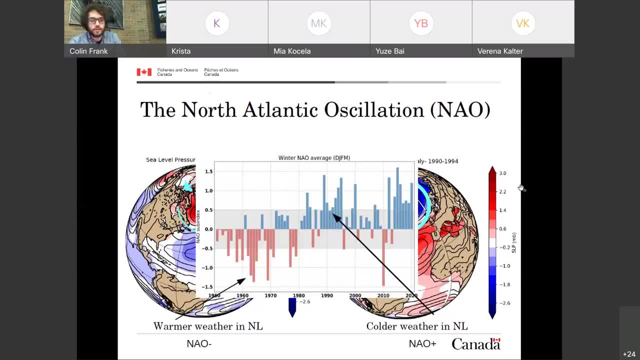 Kind of handy way to represent these changes is to talk about the North Atlantic oscillation that you might have heard of. So the North Atlantic oscillation is just constructed as a As the pressure difference between this high and the slow. So when it's positive there's a higher pressure difference, when it's negative There's a lower pressure difference. 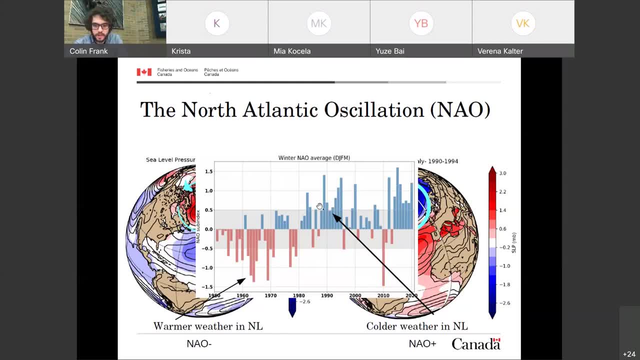 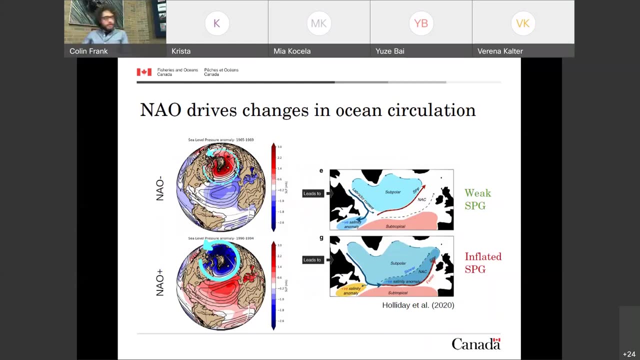 Such as in the nineties, where there was a positive, So um colder years. in the sixties there was a negative, So warmer temperature. So I'll come back to this concept later. but, as I said, These changes in the in the wind pattern can change. 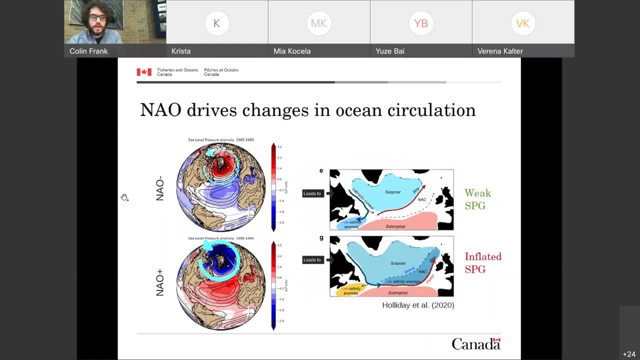 The ocean circulation as well. So in a set up where we have a negative, That would generally lead to a weaker support, Such as illustrated here, And when you have a a positive or a strong airflow, You would have a inflated support. 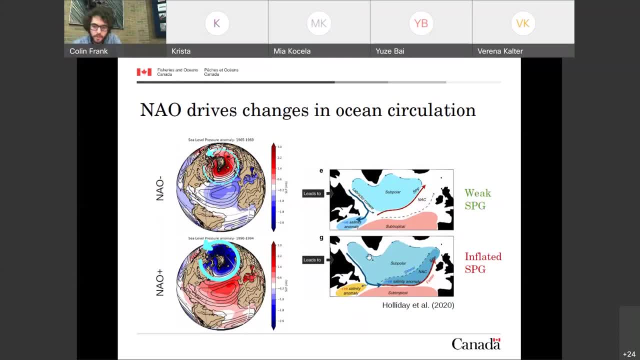 As you can see here there's a pleasure is bigger but more importantly for us, When there's a stronger airflow about the North Atlantic, the lavender current here As a tendency to be deflected offshore Compared to in a weaker support setup. 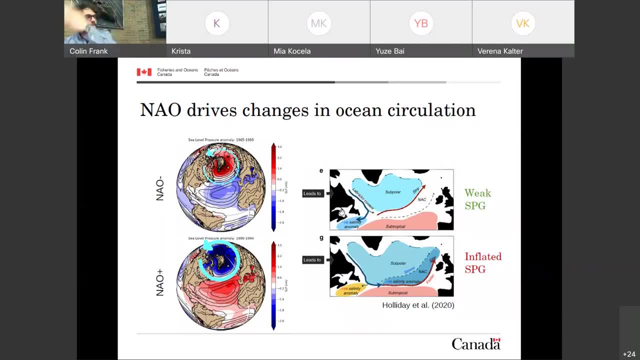 It has a tendency to loop around the grand banks And bring fresh and oxygen and water Towards the Gulf of St Lawrence and discussion shelf And this has some consequences on the ecosystem. In this paper, for example, um, it was shown that uh. 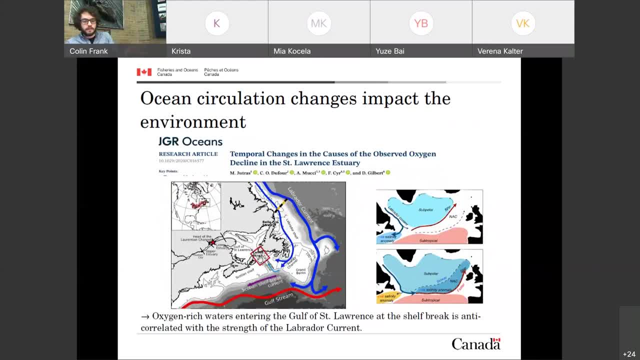 The decline in oxygen in the entering cabbage straight here Was actually well correlated with the strength of the Lavender current looping around the grand banks. as part of uh of this, for example, this uh, this setup. Same thing here, uh, in 2020, uh, there was a CBC article saying that the deep water temperature in the Gulf of St Lawrence 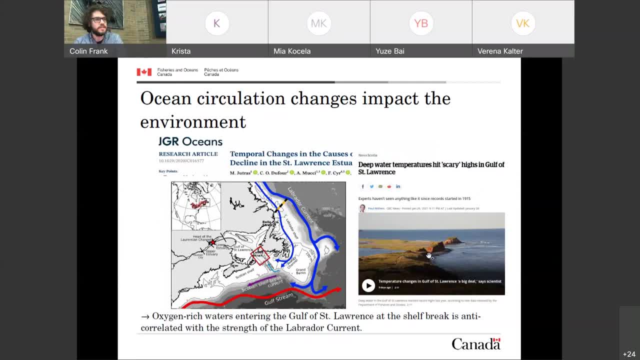 We're hitting scary highs. uh, we're talking about 5 or 6 standard deviation above the average, Something very high. this is because it was less lavender current looping around and entering Lawrence and channel here And more warm. So again, this fine balance between a different current. 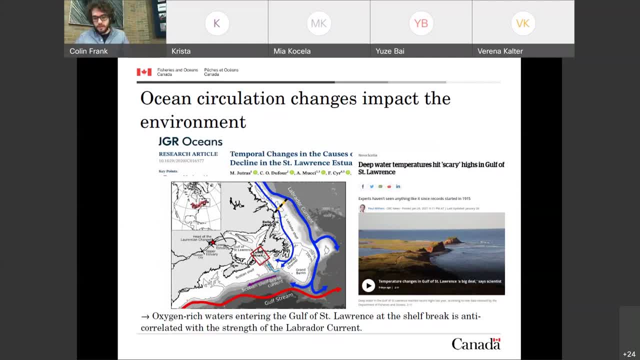 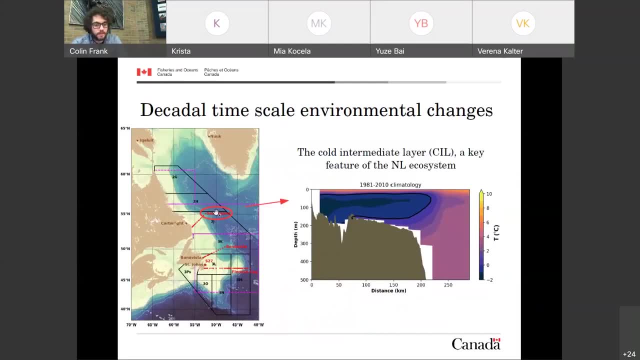 In place pretty influences the, The ocean climate and the ecosystem. Uh, same thing for the lab, Labrador or or Newfoundland shelf. and To illustrate 1 of the difference between, uh, let's say 1 period to the to the other, I I um introduce here the cold intermediate layer, or, which is a key feature. 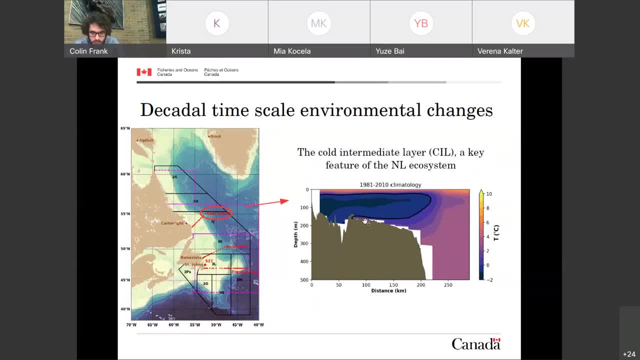 Of the uh of the analytical system, and to illustrate that I show a temperature section Along uh, what we call seal island section in Southern laboratory here. So this is 1 of our core um monitoring section. So what you see here is basically the coast is on the left hand side. 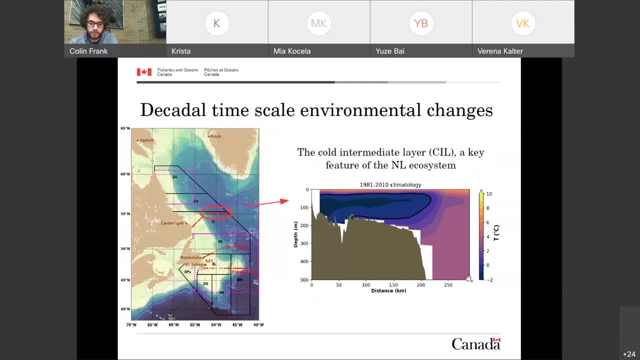 So this is 0 to 300 kilometer offshore. Uh, this is the topography. So there's, the shelf Is here and the shelf break is just here, And, uh, you can see from 0 to 500 meter. 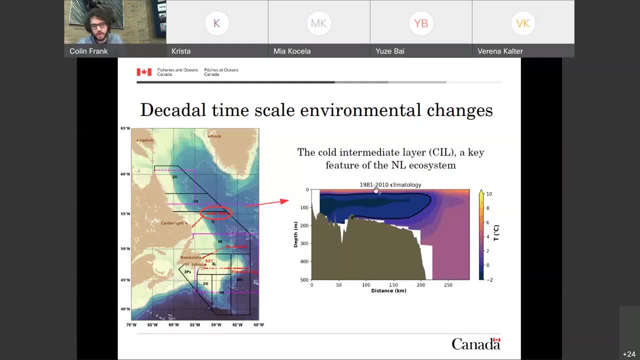 And this is the climatological value. Um, this time is the old climatology, So 1981, 2010,. but it's about the same as the new 1.. Uh and um, What you see, the dark black contour here is the 0 degree Celsius contour. 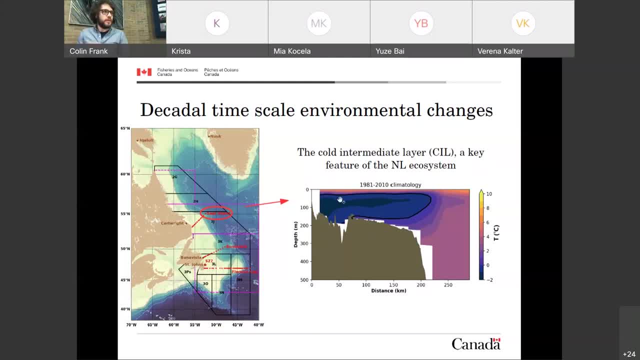 So everything within this black contour is below 0. And we're talking here about temperature, And in July- that's in Southern laboratory in July- it looks like this is a thin layer at surface of maybe reaching 10 degree, But then underneath, uh, there's a huge volume of water below 0. 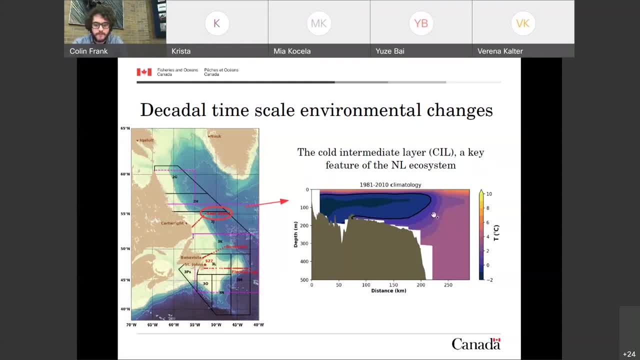 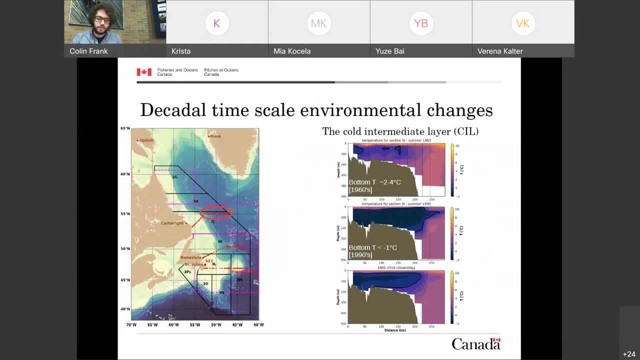 So you can imagine it is quite important for the, The ecosystem. the thing is that from 1 decade to the other this cold intermittent layer changes a lot, And I give 2 kind of extreme example here. Uh, in the 60s, 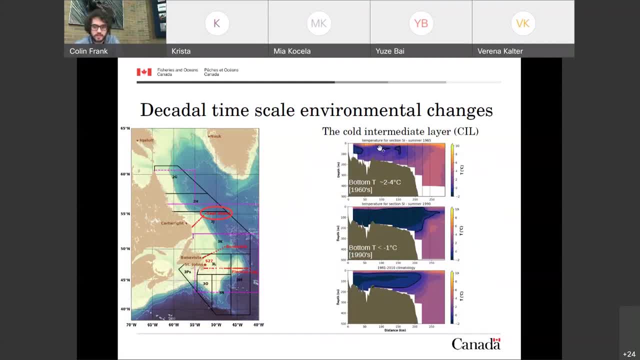 Uh, the was almost uh absent. just a little pieces here and there, Um, which also led to what a water temperature on the bottom here Between 2 to 4 degree Celsius if you look at 1990s here. 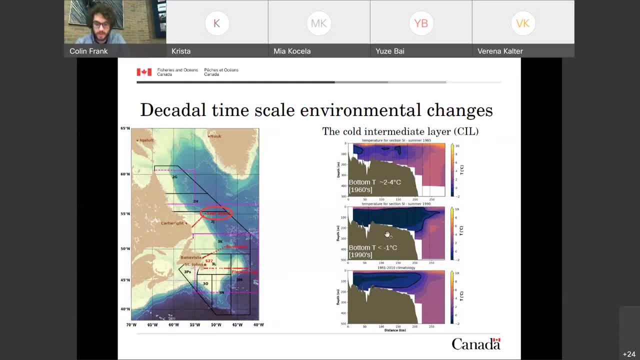 Uh, the was huge. It was also cold because this darker shade of blue here is minus 1 degree Celsius. So again, most of the water- subsurface water- in the 90s were occupied by water Below minus 1 degree Celsius in the summer, and also in the sea floor, where you have below 1 degree Celsius water on the seafloor. 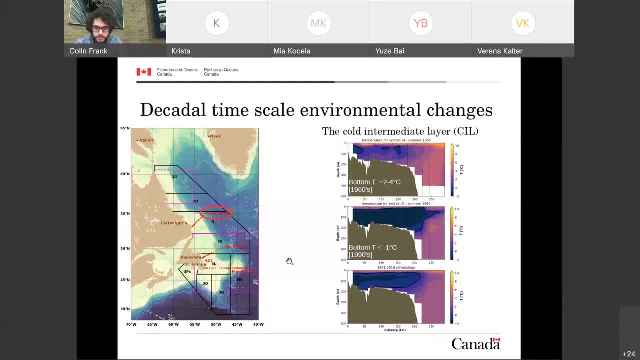 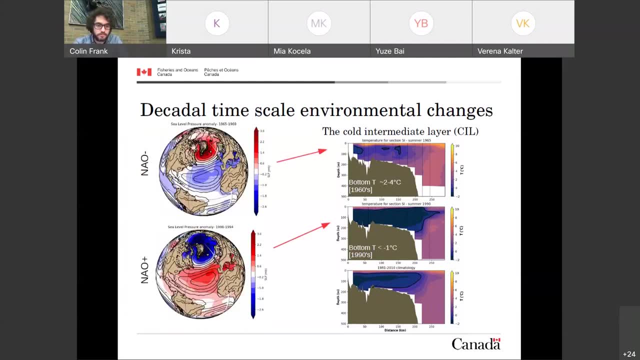 And the bottom here is the climatology that I already introduced. So, from 1 decade to the other, huge changes, And you might have guessed it, these changes are Mainly driven by, uh, what's happening in the atmosphere, In the case of a, for example, um. 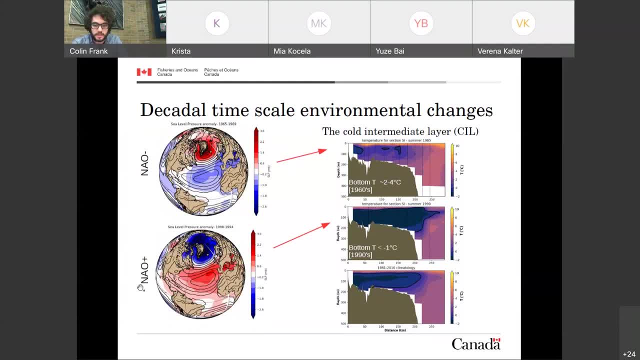 Negative set up- you would have Tendency to have this- and a positive set up. You have to note, however, that 1 year is not sufficient. You need multiple year, Multiple year, 1 after each other, to generate this whole water volume and to to shrink it. 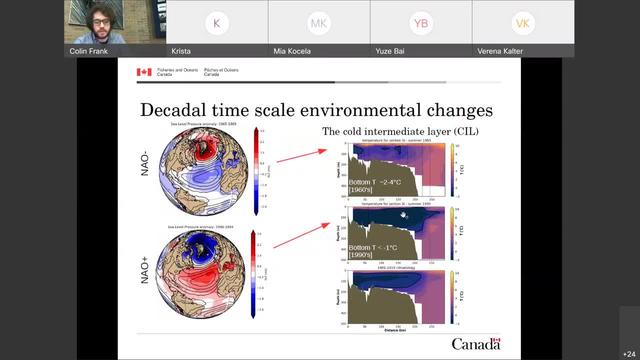 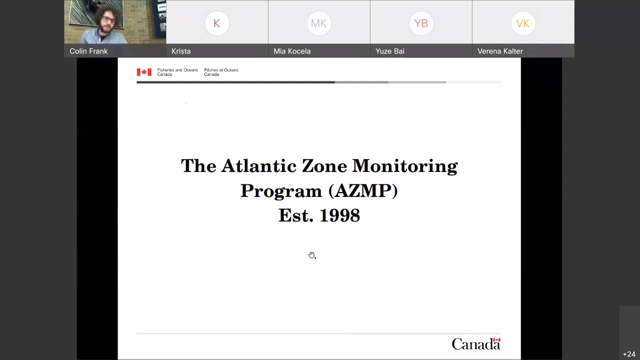 So the 1990s corresponded to the, To the collapse of the ground fish fisheries, which was a trauma for the, For, for the region here and for Most of the Atlantic Canada. so, following that collapse, um, because it was also 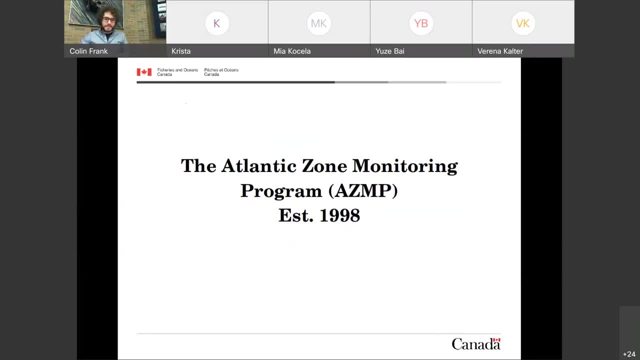 Coinciding with a period of very cold condition. the authentic zone monitoring program or was created in 1998 and this is the core, Uh well, 1 of the core aspect of my. my job is to work for this program. 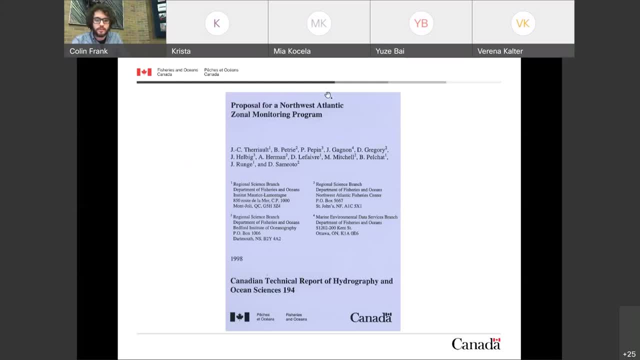 Um, so, as I said, there was a proposal for a Northwest Atlantic uh monitoring program In 1998, so that's the kind of Funding document of the funding document of the of the and in the very 1st, 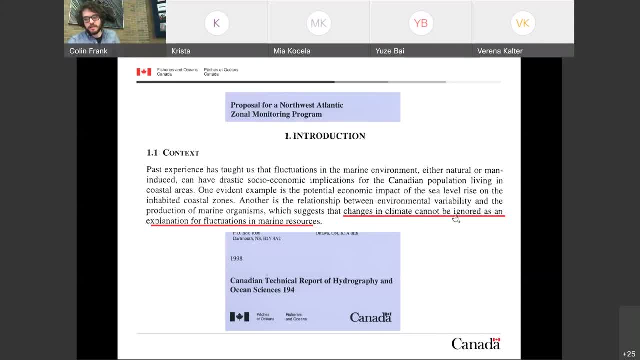 Paragraph of the document. it says that changes in climate cannot be ignored as an explanation for fluctuation of in marine resources. And it was really the. the idea of creating this Monitoring program is to monitor the environment, to better inform This management. um, and since, 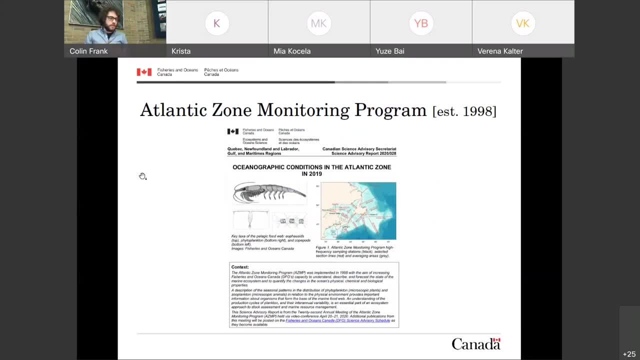 This time we produce- uh, Us, uh uh. researcher associated to the, every year a report on the oceanographic condition in the authentic zone. So this zone has researcher from Newfoundland, But also a discussion shelf here and the Gulf of St Lawrence, and not only the physics but also biology and biochemistry. 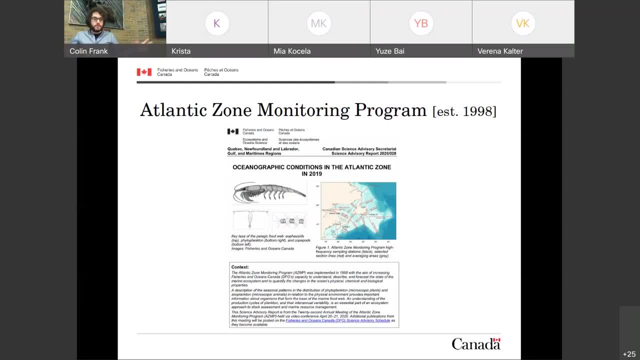 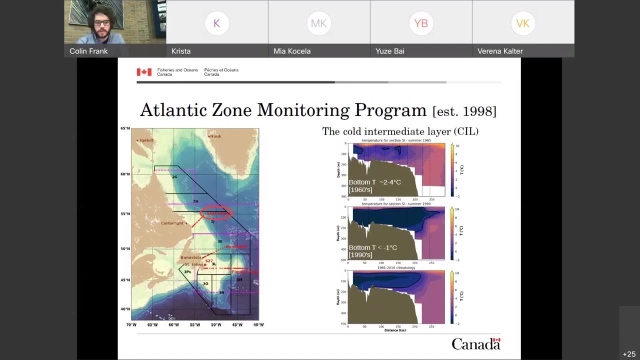 Um, uh, components. so we all Gather together once a year and we produce this report where we basically describe The ocean conditions. So, uh, coming back to uh, to this, uh, you know, kind of stuff that we can um, 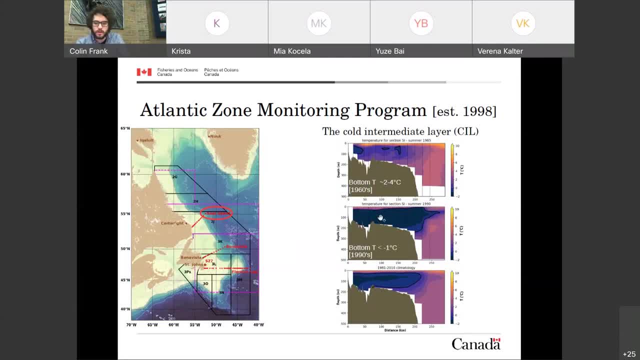 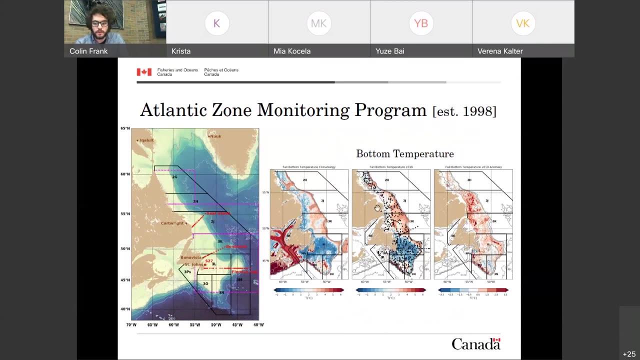 We can uh, inform, uh as part of the. so I bring back this figure where, where I mentioned that Bottom temperature here was very different from the sixties and the nineties, We can also actually measure bottom temperature since um. 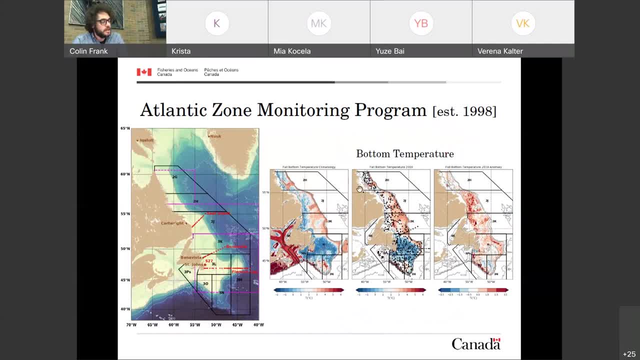 Since the the early eighties S? Uh since we have a instrument- temperature and and the salinity uh instrument on the trial and scientific trial That we use to to assess the resources. So each of these dots here corresponds to uh. 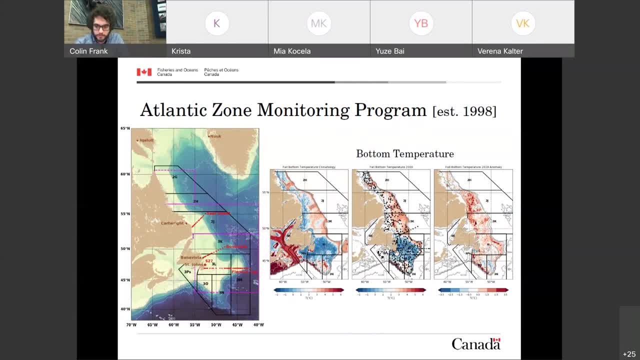 A place where we measure temperature on the sea floor. From this you can get basically a picture of what is the temperature on the on the bottom. This is for 2019, for fall 2019.. And the- the middle panel. 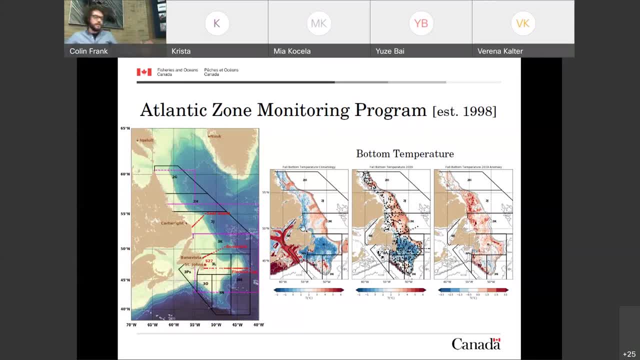 The left panel is the climatology, So the 30 year average of the bottom temperature. And every year we can contrast uh, A certain year versus the climatology and get the anomaly here. So red usually means that it was warmer than usual. 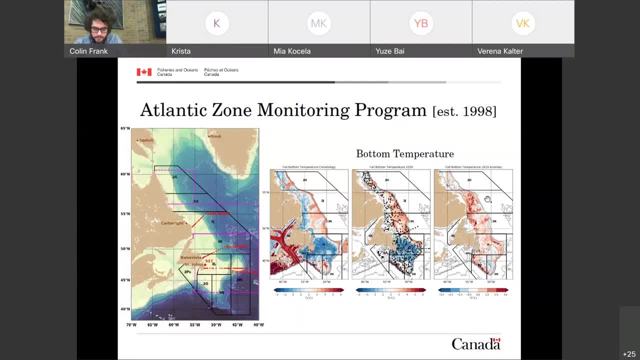 Uh, so that's for 2019.. The reason why there's 2, reason why I wanted to uh to show this specific example for The 1st 1- is to show that Bottom temperature, like any other variable, 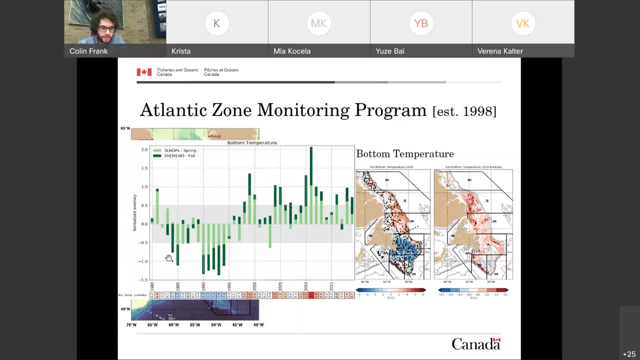 Changes on the cattle timescales. here you have a time series that starts in 1980. To 2020, so you have 40 years of data and you can see that we went through this code period in the 90s. 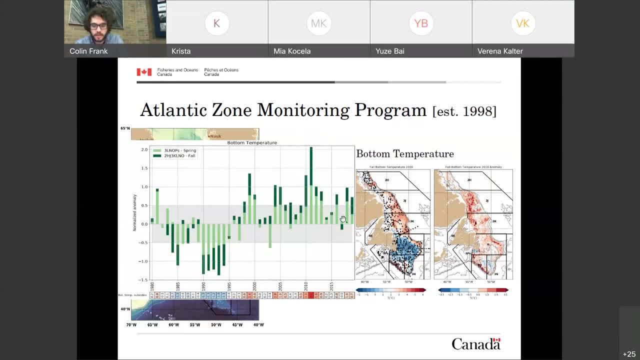 And then a warmer period that peak in 2011.. And kind of back to close to normal, although recent years were again Starting to increase. so looking at that, so that's the 1st reason that I wanted to show this. 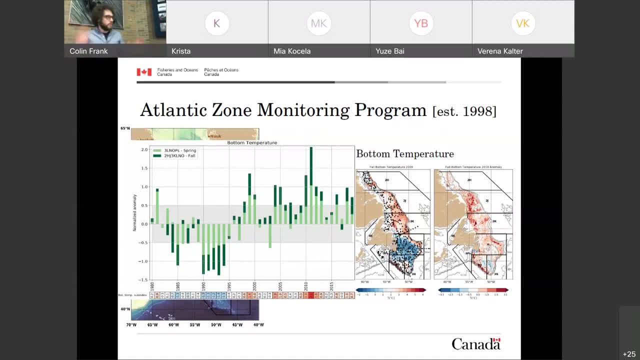 Specific example is that climate is Fluctuating. the 2nd example is: uh, looking at that, you can think: While this is enterpot and triple genic climate change, The ocean is warming, and fair enough, We only have data since 1980.. 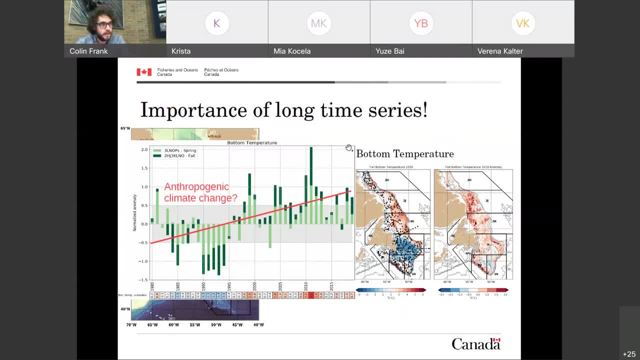 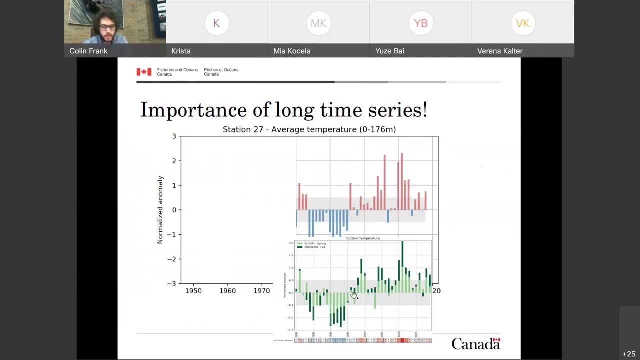 But I want to emphasize here the importance of long time series and and of monitoring programs such as the. So we don't have bottom temperature before 1980, but we do have data, as I mentioned before, at station 27, which is again one of the longest time series in canada, uh, and if we compare these two, we they. 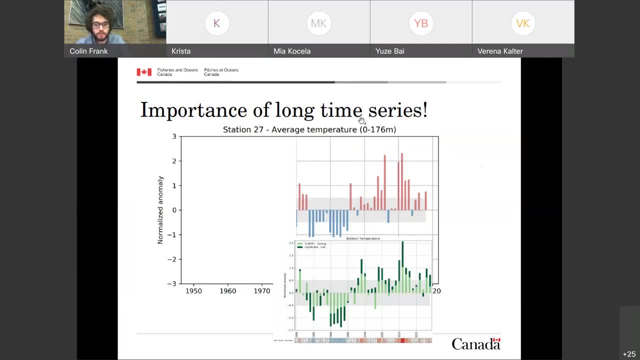 track each other very well, even though this one is only the bottom and this one is the average temperature for the entire water column. what uh station 27 inform, however, is that the 60s was actually probably the warmest period. so just looking at the zoom in the recent years, we don't. 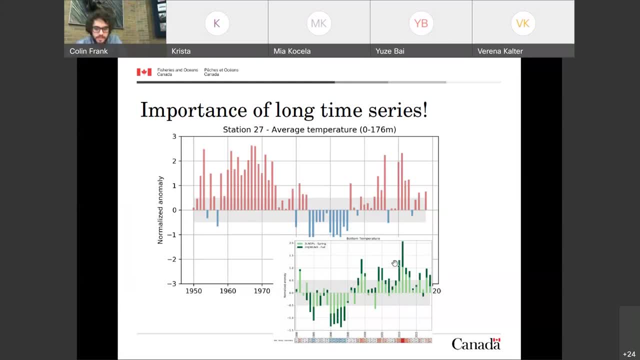 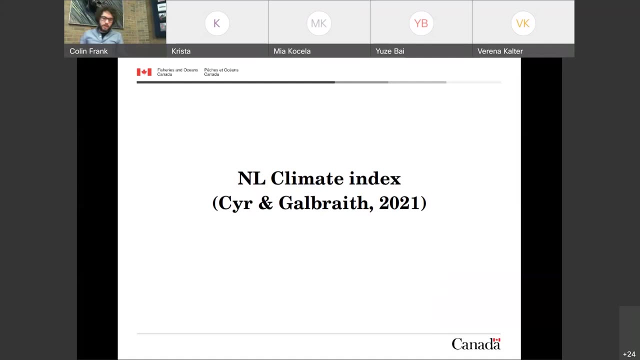 see the full picture and and actually this is part, very likely, of a natural cycle in in bottom temperatures. okay, so i mentioned that uh um long time series are important, uh, they're important to inform uh ecosystem, uh research. so in um, actually, i must admit, i was pushed by a lot of. 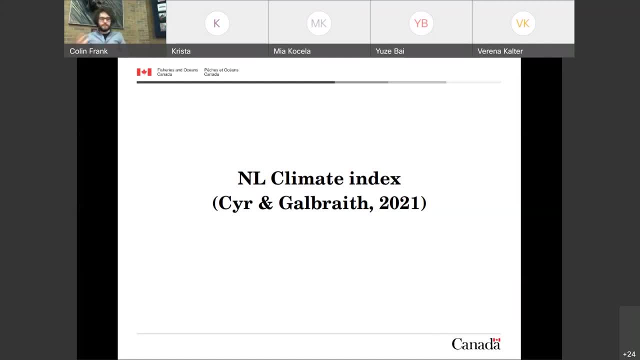 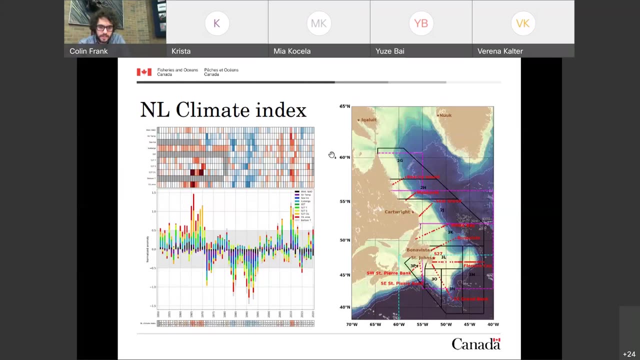 my peers to come up with some, uh, kind of simplified indices, uh that they can relate the climate to the fisheries or to the ecosystem. so last well, this year 2021, we came up with a climate index, and i will finish my talk talking about this index. so 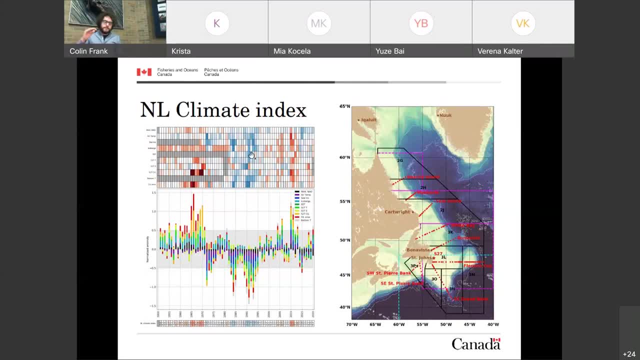 the newfoundland laboratory climate index is basically a composite of 10 different sub-indices. these sub-indices are- i don't know if you can see from the from there, but the winter north atlantic oscillation or like that- the atmosphere set up in the winter, then the air temperature at five sites. so nuke in greenland. 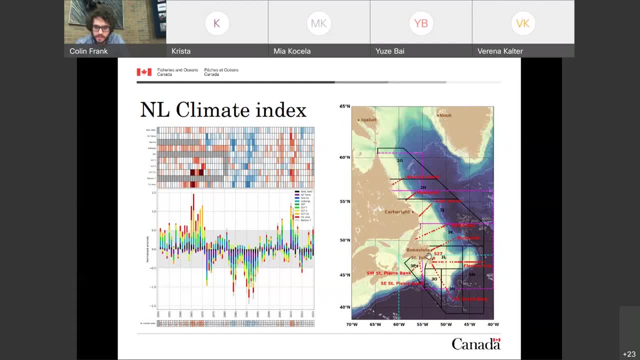 eucaluit, baffin island, cartwright and labrador and bonavista, st jones, uh the sea ice in three boxes, so um in purple here. so northern labrador, southern labrador and newfoundland, the number of icebergs uh crossing a line here at 48 degree north then from station, uh the sea surface. 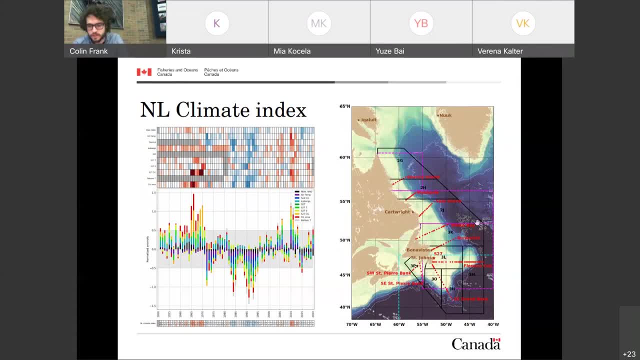 in these black boxes here that are the nafo divisions. uh, also from station 27 i have temperature, salinity and the minimum temperature of the cil, so the coldest water we can get. i also have the average the, the area of the cil over a hydrographic section, so seal island. 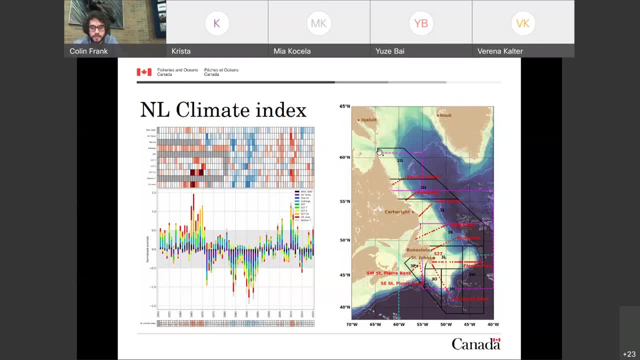 bonavista and flemish cap and finally the bottom temperature in these nafo divisions again, but clip at, the shelf break. so each row here represent one of these sub-indices, uh, color coded according to whether or not it was warm, red or cold, blue and. 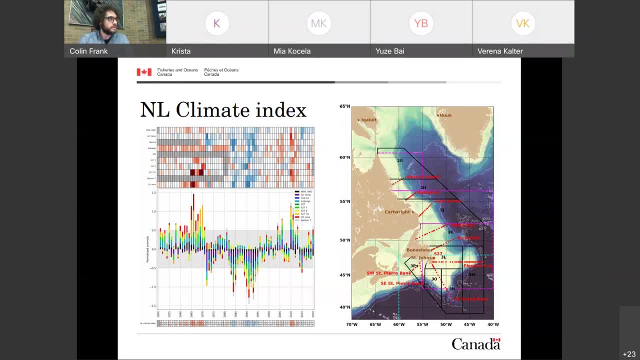 the the deeper the color is, the more standard deviation above or below the average we are. so, uh, and when it's gray here, it's because there's no, there was no data, for example, the time series started later, so all these uh, basically lines are collapsed into a 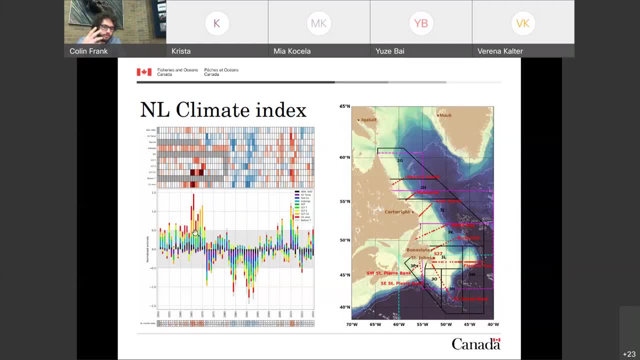 uh, a stack bar plot here to to visually better see fluctuation in the in the climate since 1950 and the average of of this um, of this index is again presented at the bottom here, where is the average of the 10 time series. so that is the, basically the climate index. 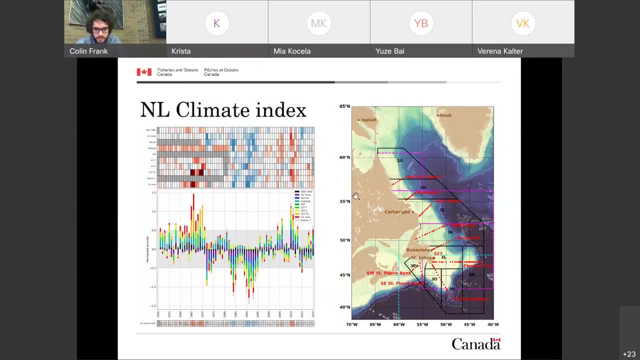 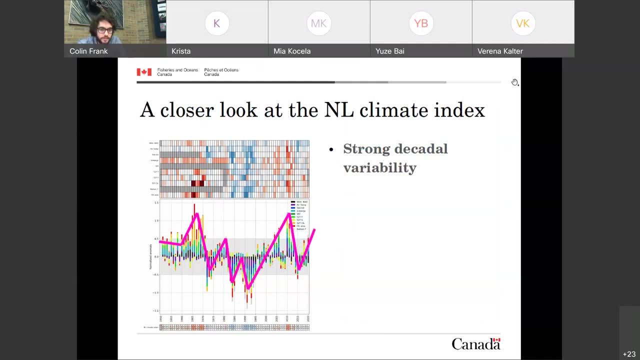 um, and again color coded according to the stem. so we can say, uh, let's have a closer look at the nl climate index. so we can say many things. first of all, as i said before, strong decadal variability of the, of the climate in the flora and labrador and this climate, this climate variability, is linked to, as i said before, this. 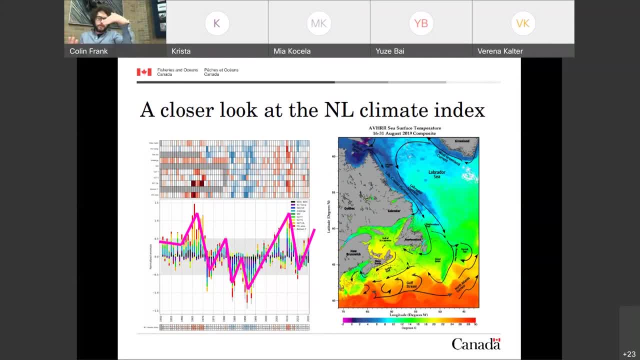 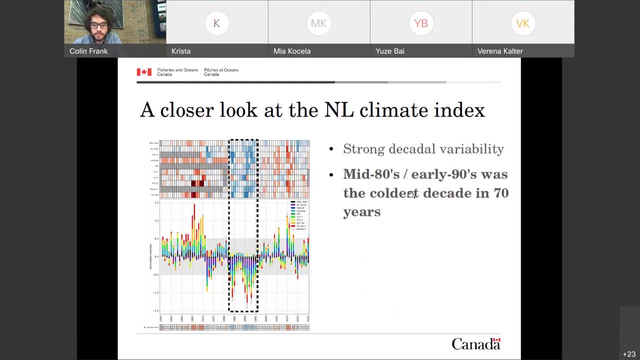 kind of fine balance between the water coming from the north and water and warmer water coming from the from the south. we can also say that the mid 80s, early 90s was the coldest decade in, uh, the last 70 years. this is pretty clear here if you look at all these blue cells here and all these- uh this bar going down. 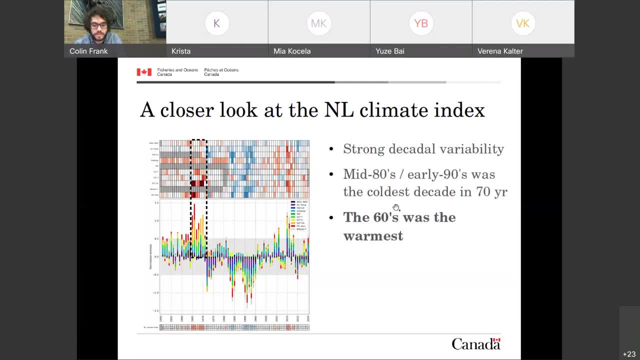 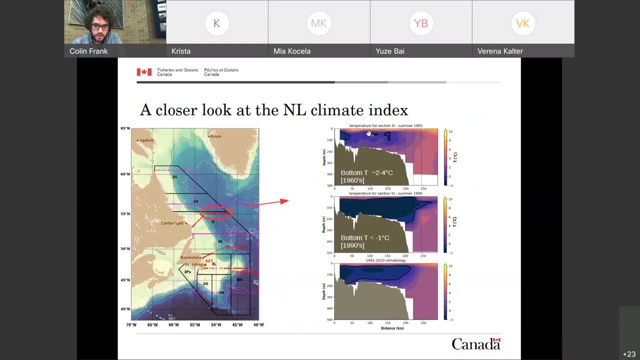 at contrary, the 60s were the warmest decade, uh, as you can see here and here it was highly driven, uh, though, by the cold intermittent, a very warm, cold intermittent layer. so, as i said before, so that was the 60s, where there was almost no cil. 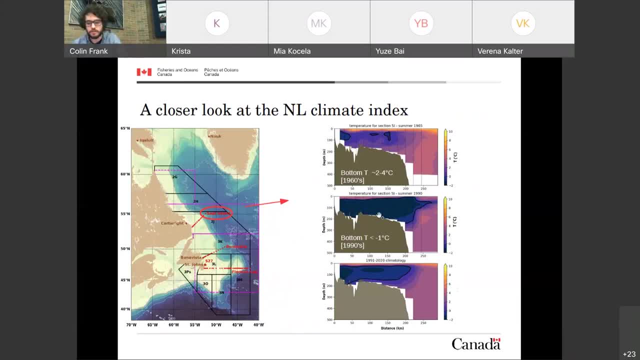 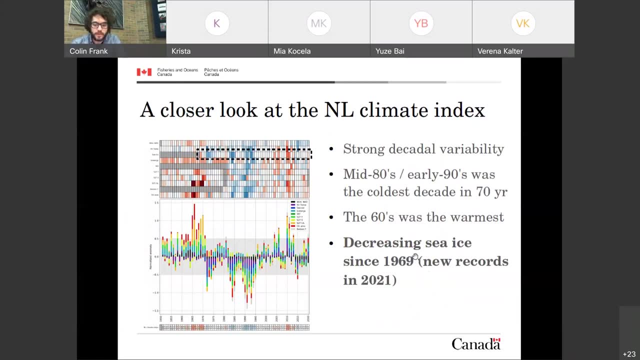 versus the 90s, where it was much, much bigger. uh. also, we can see uh decreasing cis uh since the beginning of the record in 1969, as you can see here. so we're a lot of blue. blue means colder and we slowly warmed up, uh, with some. 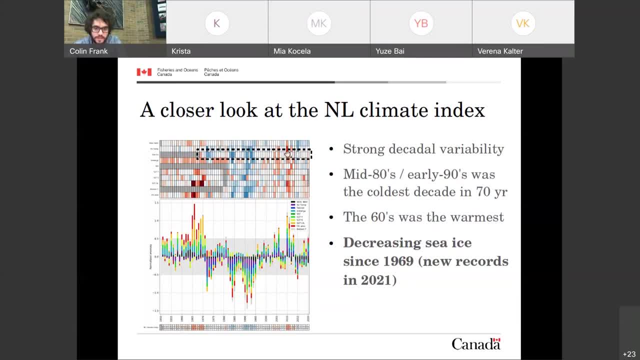 there was a previous record in in 2010, but actually 2021. that is not there. uh, we're still in the 20s. uh, so we're still in the early 20s in the middle of this time period. i just wanted to once again. 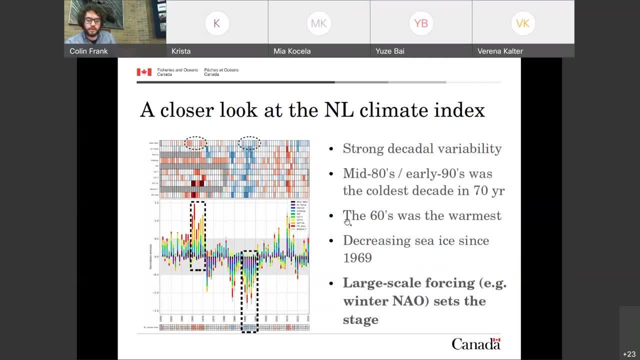 give you a little bit more detail about how this works, because what this does is it? it と set the new record for the next half of the year and at the end of the year. and uh, the other way it's a new record. uh, as i said earlier, for this one it does the same thing that it does for the. 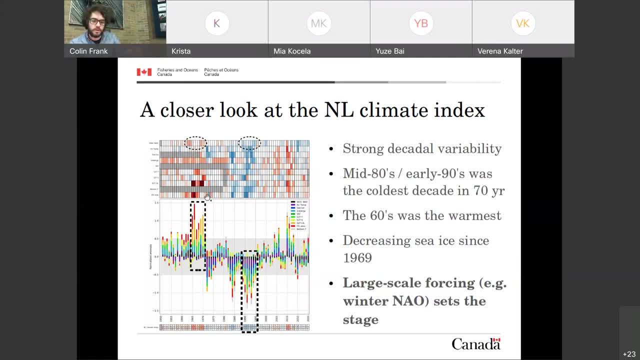 upper end of the year. it's base, and here it's a little bit bit of a panoramic that makes it a uh nice, a little bit uh big scale record. now let's look at the large scale. positive nao will lead to a cooler climate. so there's anything, many other things. i, i, yeah, as 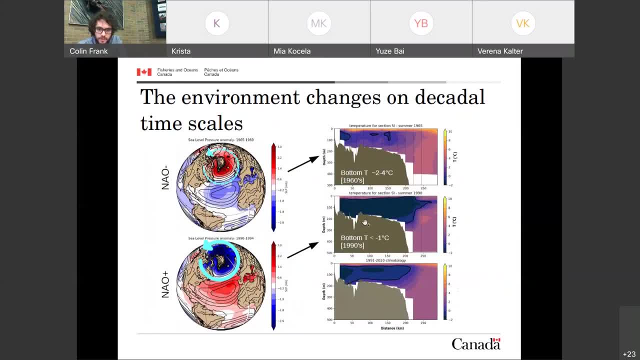 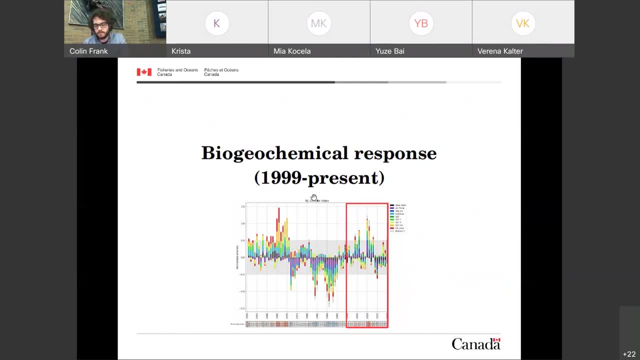 i mentioned here. so negative nao leads to this, positive nao leads to this. so there's many other things i could i could say about that, um, but i i'll switch to something else now, which is the biogeochemical response, and we can only talk about biogeochemical parameters since, uh, the 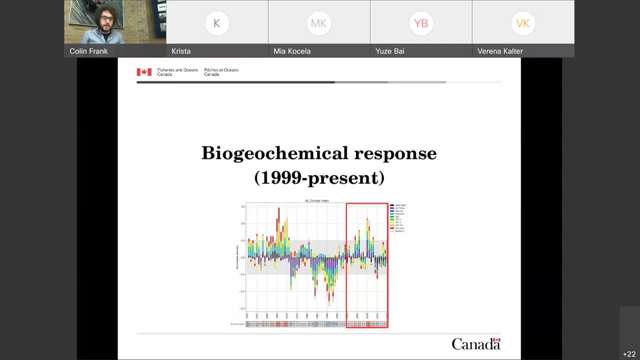 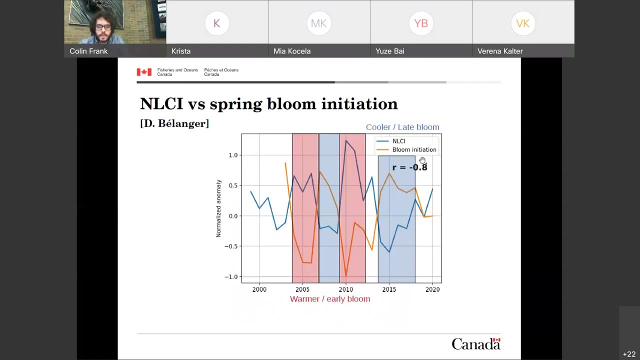 introduction of asnmp in in 1998, 1999, where we started this kind of measurements on a regular basis. so we'll focus more on the recent period here and i will just give you two examples of ongoing work. um, uh, where i what? what you see here is a plug of the nlci, so the nl climate index. 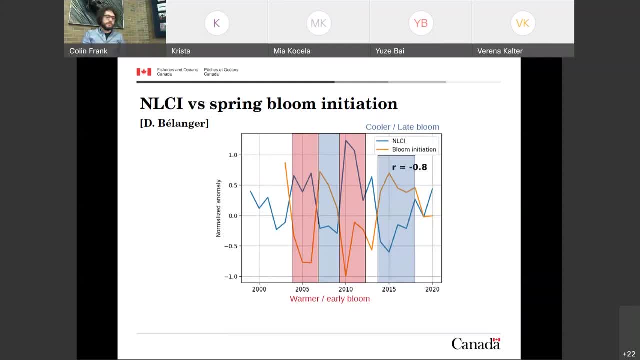 versus the timing of the initiation of the bloom. so in blue you have period of warmer climate that are delineated by red bars here and the timing of the bloom for the entire region in orange. so what we see is that when we have a warmer climate we have a an earlier bloom. so negative anomaly: in the blue means earlier and vice versa. so 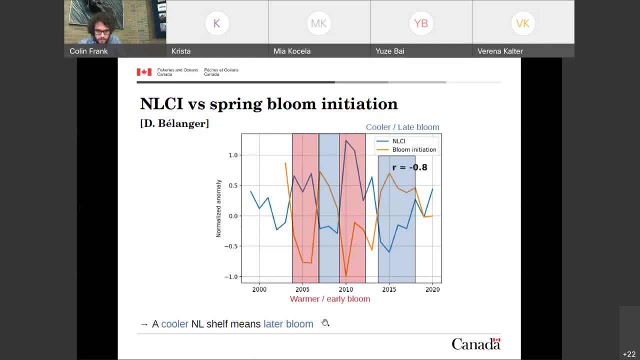 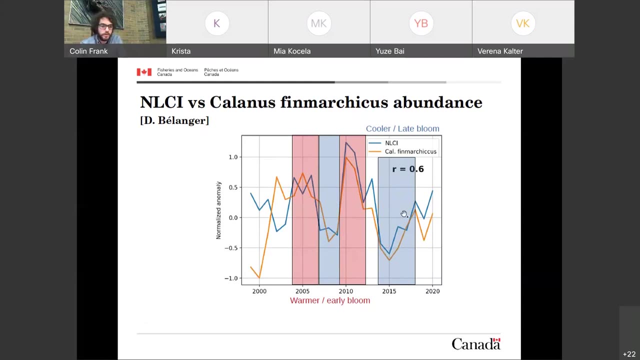 in other words, cooler nl, later bloom and vice versa. it's not really surprising. but what is surprising is how much predictive power we have with the climate index to the blue initiation. we also have a good predictive power of the climate index on the abundance of canonus from archicus, which is one of the key taxa for um for the ecosystem. 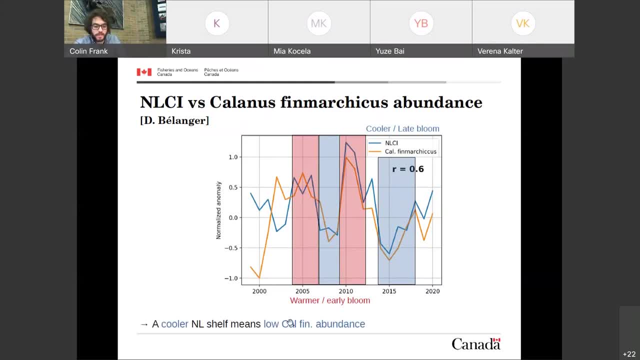 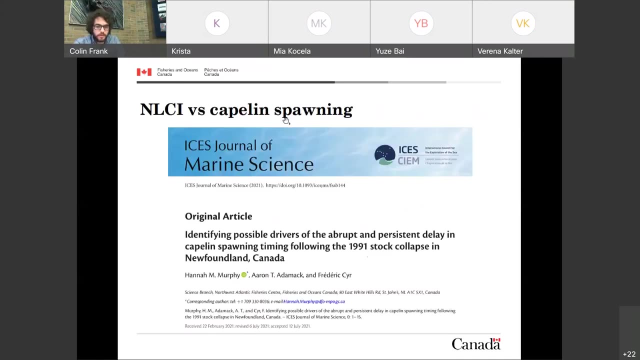 here. and then same thing: a cooler nl shelf mean lower abundance of kelvin and vice versa. so, as i said, this is very, very fresh work that i um added to my presentation. um, i give another example of stuff that has been published earlier this year where the 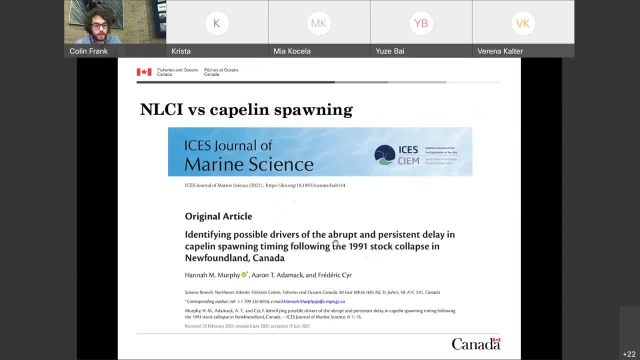 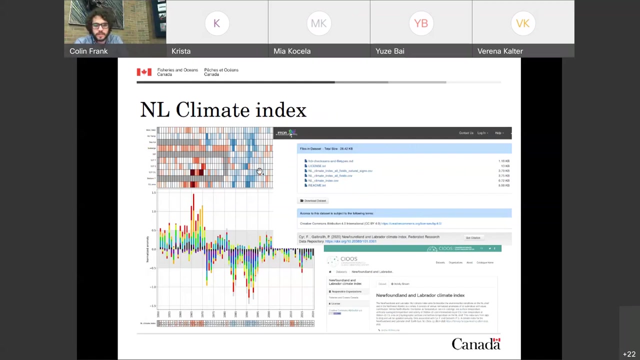 nlci, the nl climate index, has a good predictive power on the timing of the spawning of cape land. um, it was not in terms of the environment parameter that was the best parameter to predict the timing of the spawning. so, uh, that's, uh, that's it for me. uh, so this, i really wanted to introduce this climate index. 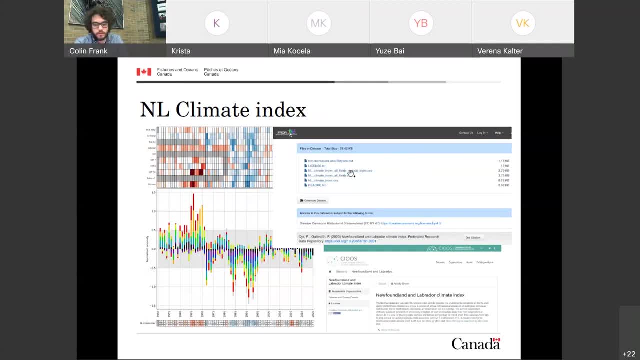 because it is um openly accessible. so if you if you are doing any ecosystem study and you want to have a broad overview of the climate in newfoundland labrador, you can have a look um it is available on the frdr, so federated research data repository. 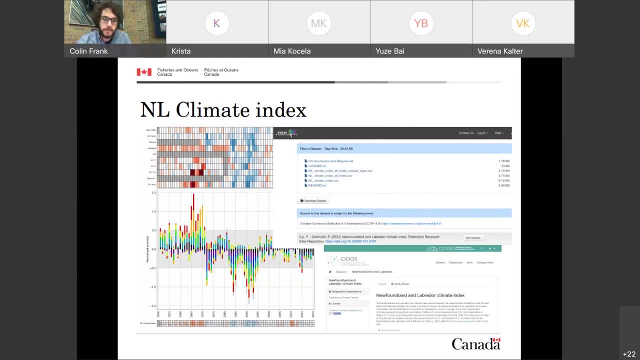 so if you google nl climate index, frdr, you should find it. it's also available on the um ceos atlantic posted here at mi um in the repository. you'll find the climate index itself, so a single time series, but you also find all the fields. so the 10 sub indices are there, so you can. 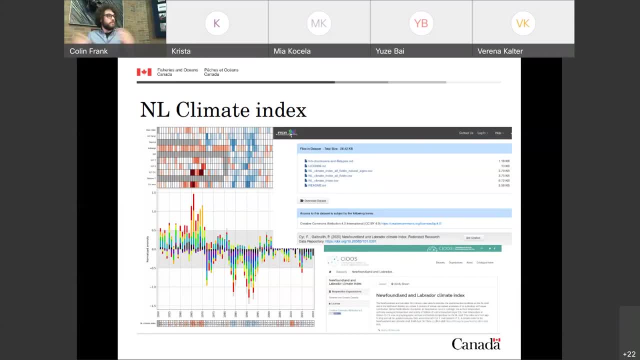 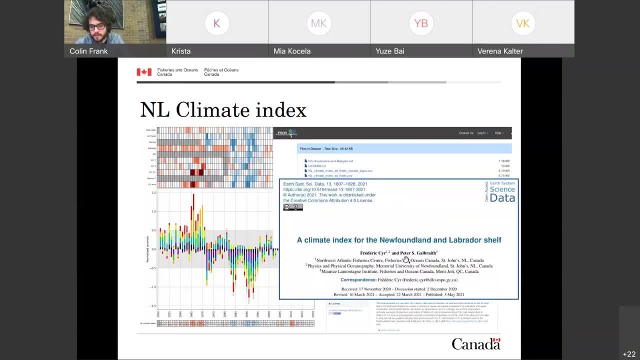 basically make your own climate index by cherry picking the units that you're interested in. uh, and finally, there's a, there's a paper that explains basically each of the sub indices, uh, and, and give basically uh graphs of all the parameters and what, the, what, the, how they, they evolve over. 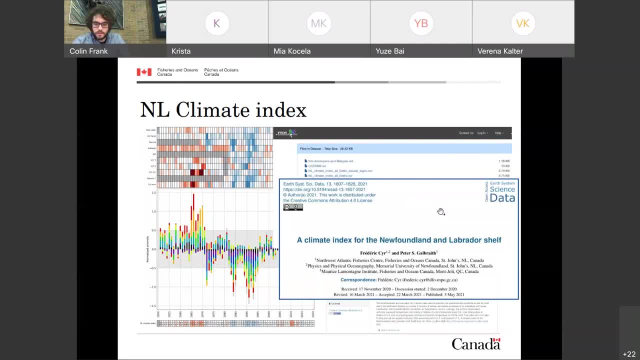 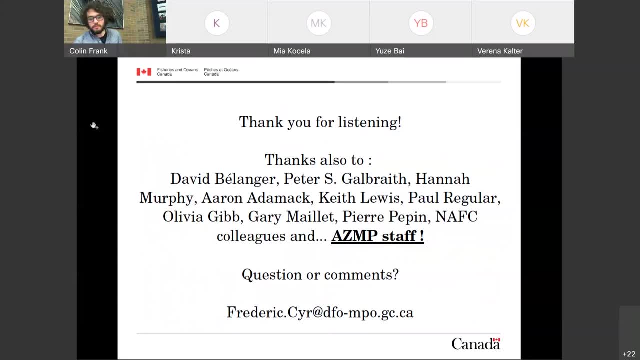 the last uh, last few decades. so that's it for me. uh, thank you so much for listening and for being here and uh, yeah, so i i acknowledge your uh help from many uh many uh colleagues that helped me brainstorming with this uh, this climate index, but i also really want to thank the all the asnmp staff. 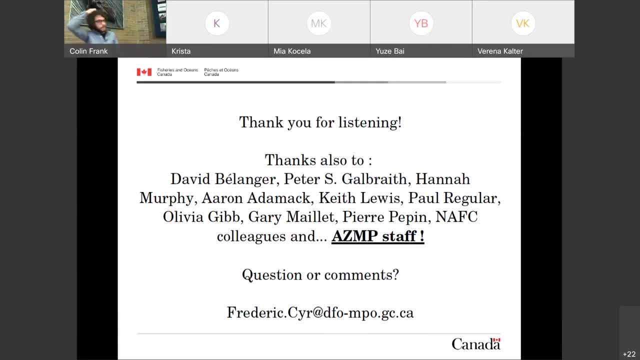 that make this possible. so thank you, and can anybody have any questions and i'll i'll feel the questions online. yeah, you can stay in the camera. we're still trying to figure this part out, that's good. yeah, it's used to in person anymore. yeah, so if anybody has any questions online, go ahead and just raise your hand. 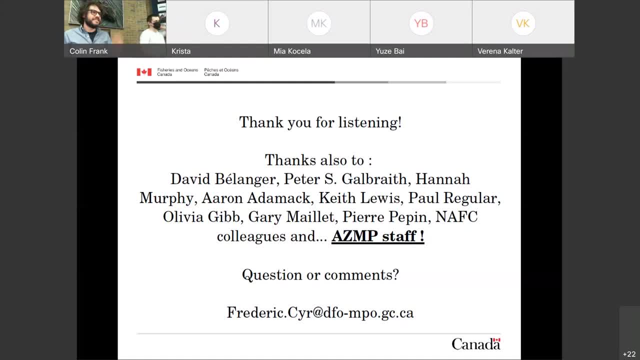 and you can raise your hand all right, turn the right hand about on yes. so should i repeat the question? maybe, uh. so the question is if, uh, all sub indices are equally weighted in the climate index and the answer is yes. so i mean there's many argument to. 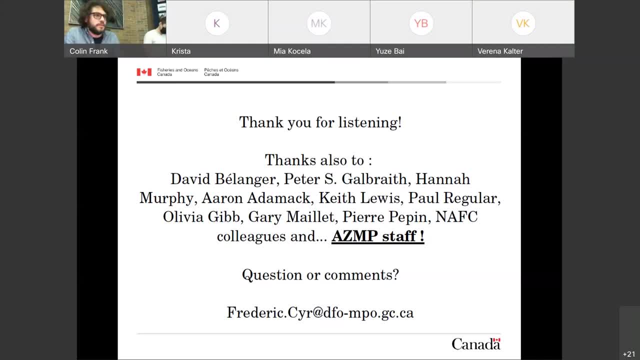 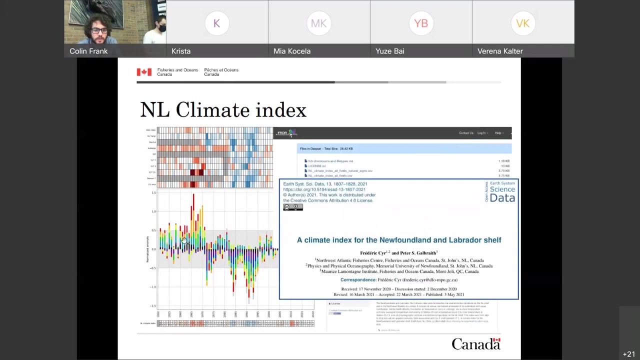 important than sea ice or bottom temperature. but, uh, there was no really good argument to how to weight this, so they're equally weighted. but then again, because i provide them all, one person can decide to weigh them different. yeah, yeah, we're the last. yeah, yeah, yeah. in recent years, yeah, in 20, since 2012, there was an ongoing positive phase of the nao, so positive. 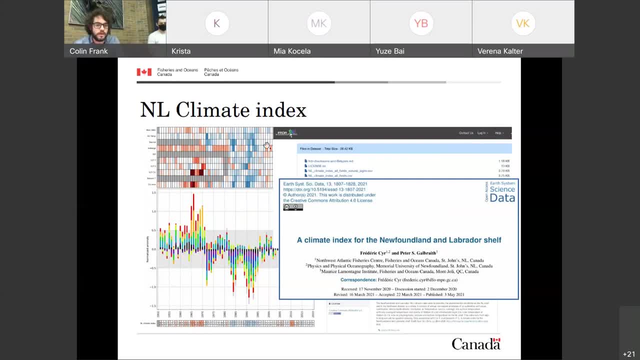 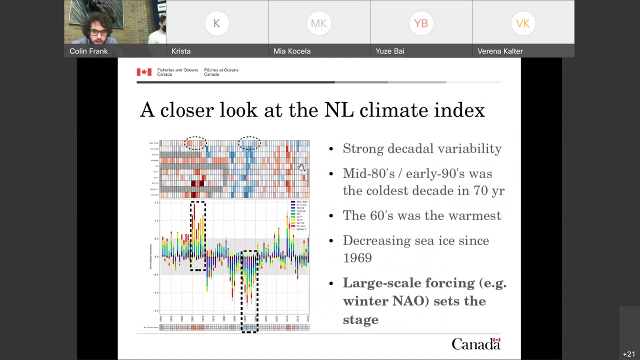 means cooler water, and your question is why? yeah, yeah, yeah, that's a good point. uh, actually there was some uh. there's different reason for that. there's the choice of uh, of uh, maybe i should, you can see it all now. so there are some uh, some blue that you can see, uh. 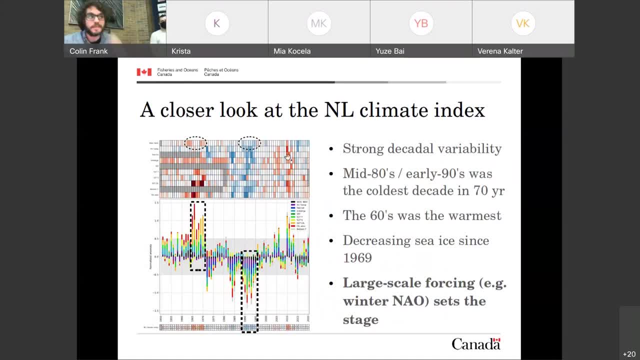 the sea. ice and iceberg were red, so it's something with ice. so, um, basically, there was an ongoing positive phase of the nao that really looked like the one of the 90s here, but the response of the was not the same, or the response of the environment. uh, we think it is because of 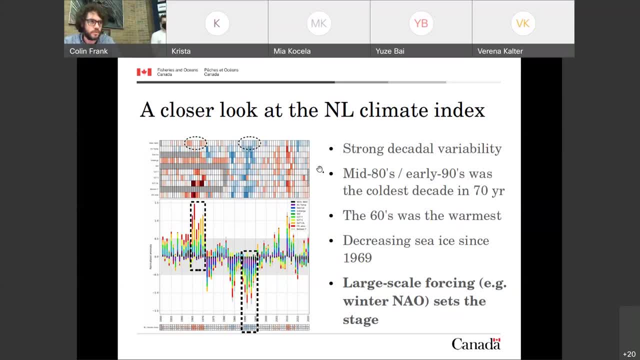 this is the anthropogenic climate change signature. so winters are milder, so sea ice is still decreasing, despite of a warmer condition, um and also sea surface temperature, because sea surface temperature is is mostly um, mostly corresponds to the summer conditions and since the atmosphere seems warmer in the in the summer, then the thin layer gets um, gets uh, warmer than than usual. 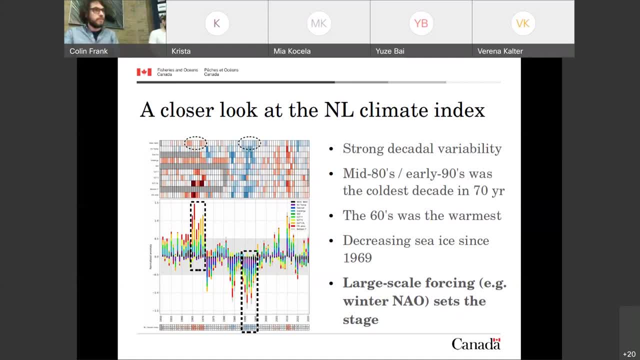 but if we look at the cil, for example, that is the leftover from the previous winter. the cil was actually cooler in a recent period as a as a consequence of the exposed the, for example. here you see negative the cool cil in response to this really cold annual. 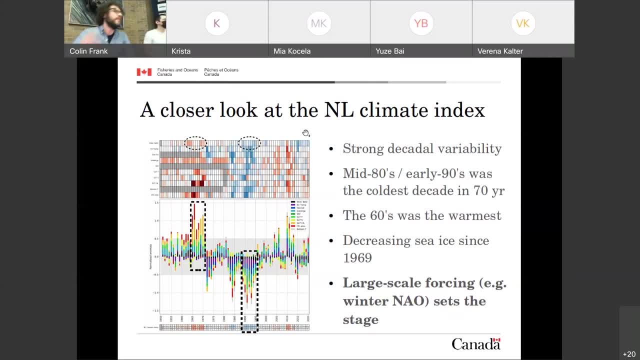 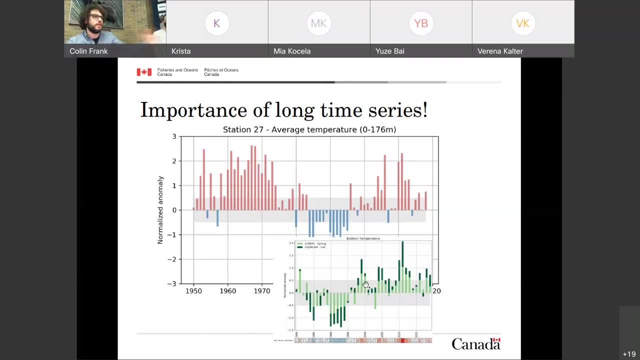 on. basically, baseline is basically the pre-collapse in the 80s, And this figure showed that actually the 60s was one of the warmest period and something we never take into account, And this is specifically something that I've been hammering over many years since I started. 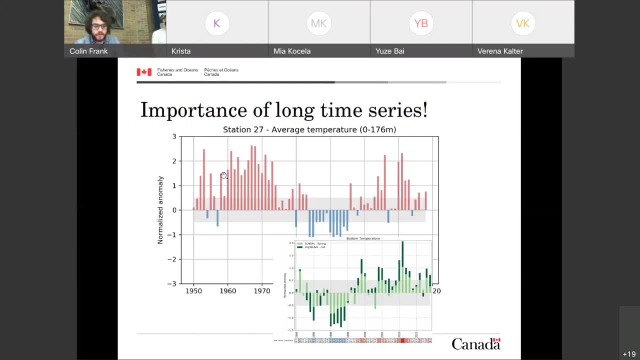 at DFO. For me this is mind blowing- that the 60s were the warmest period in the last century, basically. So was it possible that we're a bit biased when we think about our baseline? What I think- and again, this doesn't involve DFO, it's a personal interpretation, right? 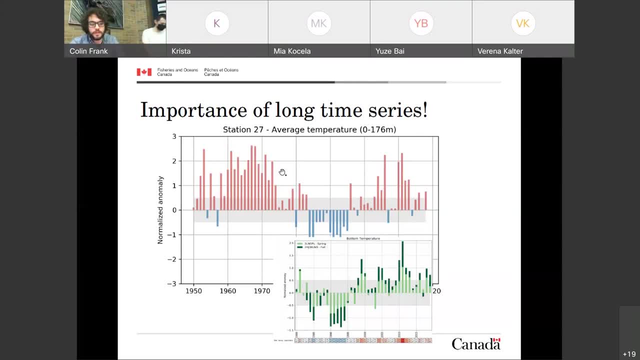 now, What I think is that when we're fishing, a lot of The industrialization of the fishery started in this period, where it was potentially an anomaly in the last century, And if we industrialize our fishery- and we had record fishery, but yeah, this was based- 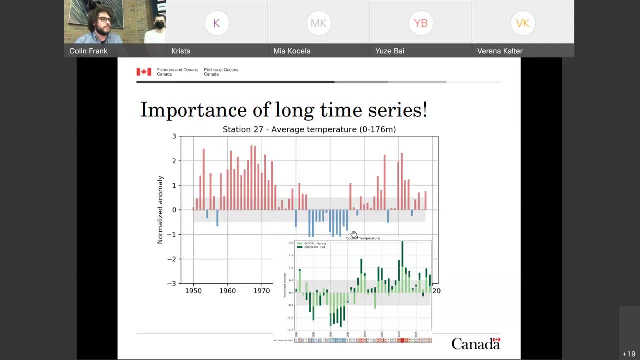 on an anomaly And then, once this anomaly was gone, then the ecosystem responded to that: Okay, So we basically kept the fishing pressure to something, but we kept the fishing pressure as high and it was there. So that would be my hypothesis. 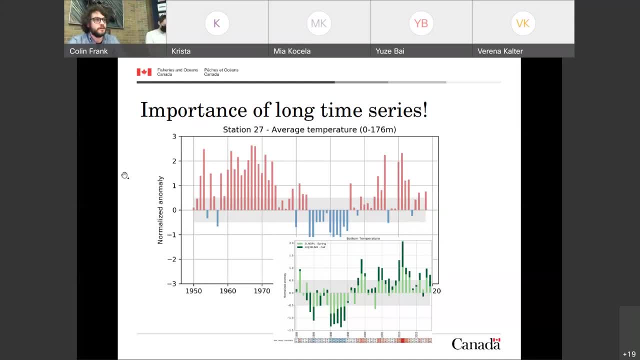 Not hypothesis, but my analysis of this. but yeah, again, it's a completely personal analysis. If we can hear you, can you hear me? Can you hear me? I can hear you. Yes, yes, Can you hear me? 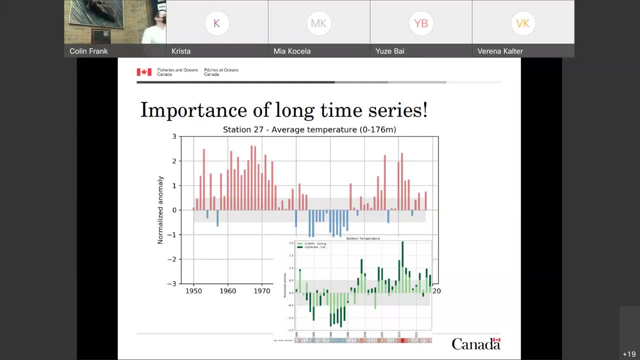 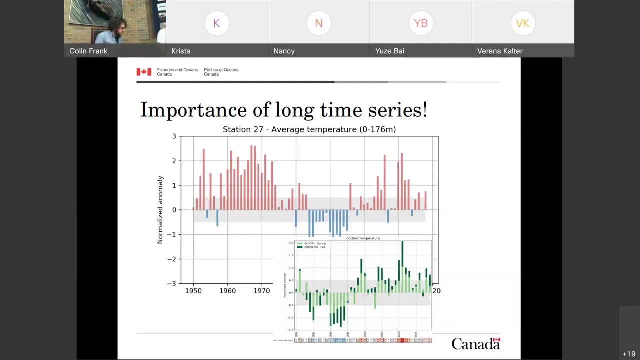 All right, thanks. Um. thank you for the presentation. Very, very interesting. Um, I was wondering if, in the data, if there's a way, or if you're able to determine transport through some of those um trends. 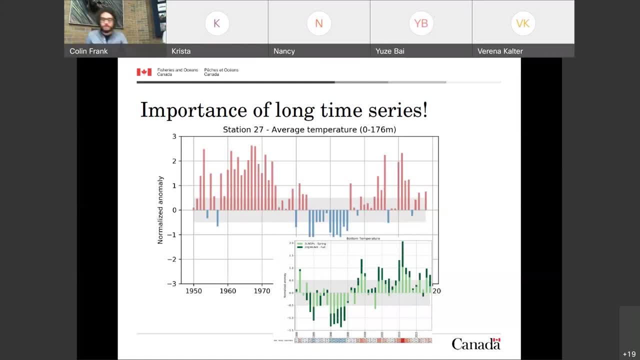 Yeah, I mean this is That's a good question. I mean we- um, there's a lot of paper that I've been trying to compute just traffic transport from a historical transit. What I've heard- I didn't try myself, What I've heard is that it's quite difficult because of- uh, 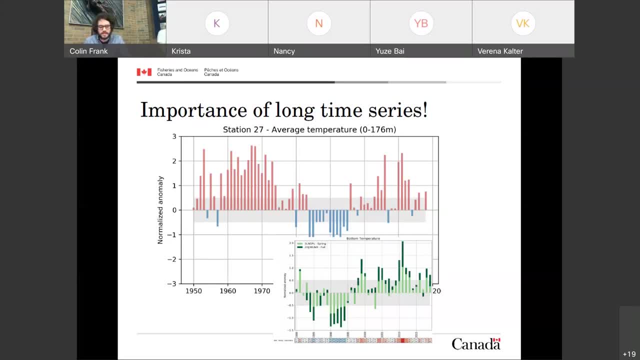 Of the, basically the, the, The title aspect and the variability- uh, high frequency variability of the uh the transport makes it very difficult Uh. but yeah, again I'd be happy to uh to try that. I know our colleagues, and then just 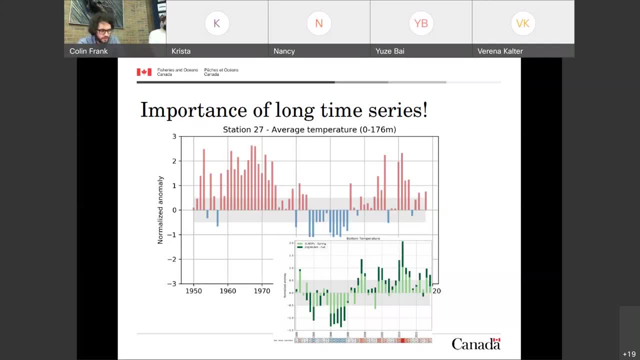 Sorry, I didn't. I don't understand, but yeah, I think our colleagues- Steve also- is trying to Try to do this. recently I had I had 1 more question, Fred, if you could. um, I was wondering if 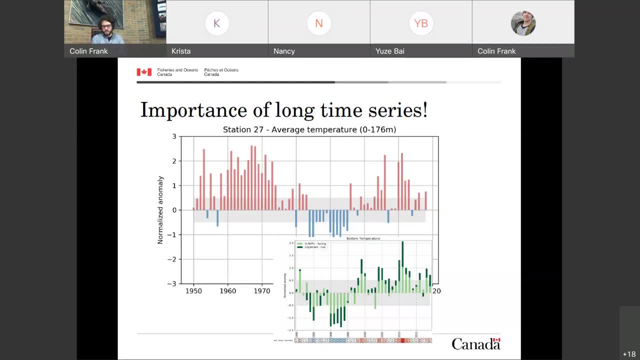 I mean you're looking at your work in the connection um Between the climate index and the capelin spawning time. Have you looked at the results for this year, I think? if I remember correctly, the capelin did spawn earlier than in the past few years. So I'm just kind of curious what how things are looking. Well, I can see it matches. I didn't check the details because, again, 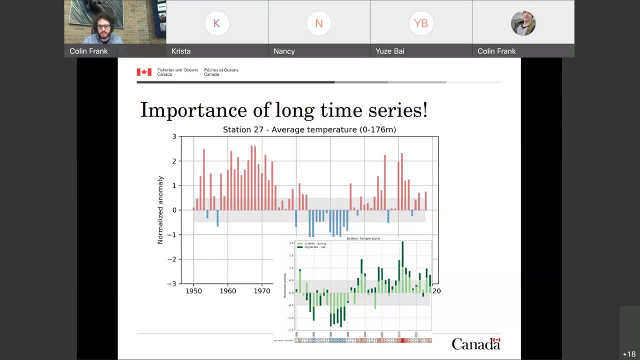 It was kind of a 1 year where the After like 30 years being delayed, the capelin came back to almost what it was before the collapse, But 2021 was one of the warmest year Um in a long time, at least since 2010.. 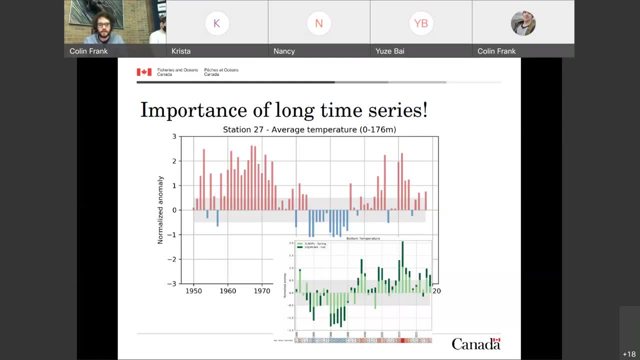 So yeah, this year is definitely an outlier. So yeah, warmer climate, we came back to earlier spawning, so it matches Cool. thanks, Fred. Do we have any more questions? Oh great. Do we have any more questions? Oh great. 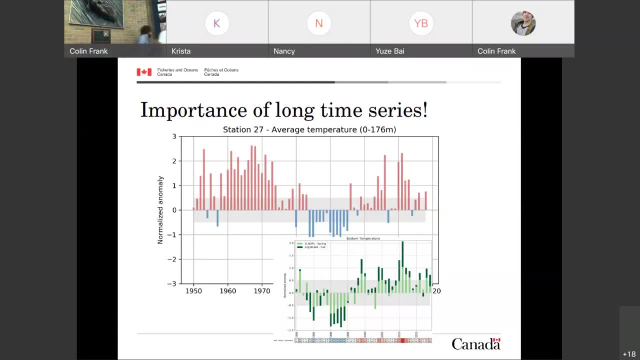 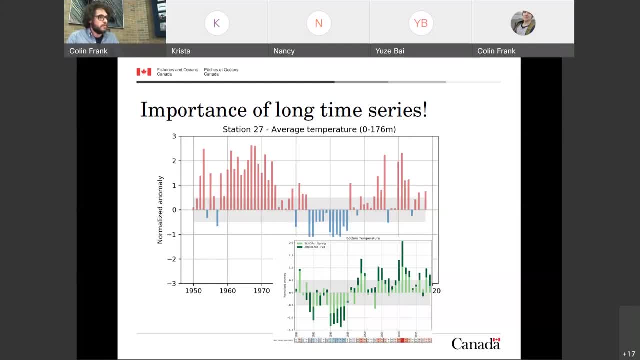 And the answer is –. the short answer is yes. The more complex answer is: I'm not sure if it's, I mean, worse now than it was, for example, in the 1960s, But, yeah, In the recent years. yes, there is definitely a freshening that we see. 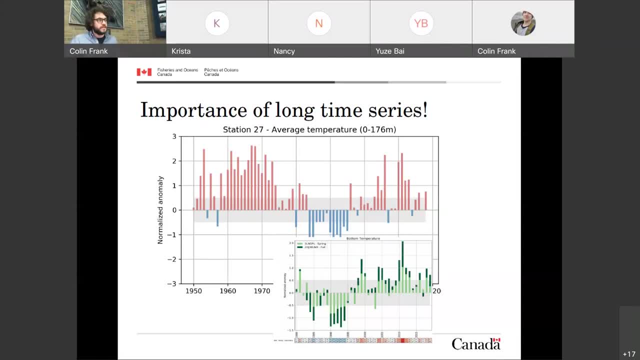 But in the recent years, yes, there is definitely a freshening that we see. not sure if it's because the arctic is melting or because of this kind of a nao pattern that brings more or less fresh water from the arctic because the the arctic acts. 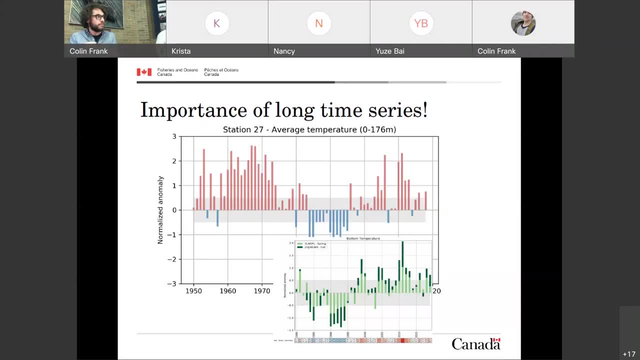 acts as a buffer, also for fresh water, so sometimes it retains water for a few few years and then you release it afterwards. so i'm not so sure, but yes, we see a freshening over the recent years. second one is that if there's potential for forecasting the ocean conditions, 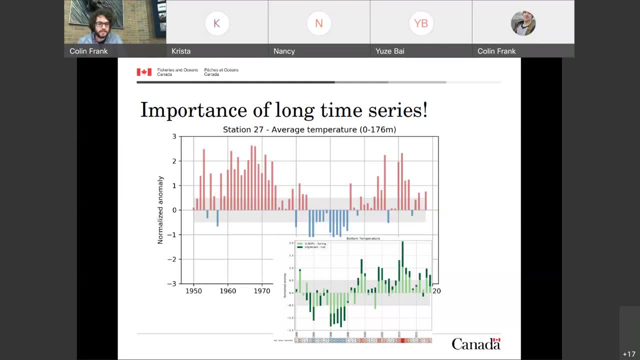 um, yes and no. and the sun? if you just look at this figure, you can see that these are slow cycles, so, of course, you might have one anomalous here once in a while, but i think we can forecast them because these are our cycles. uh, so definitely, we reached the peak here around 2010, 2011, and now we've been cooling. 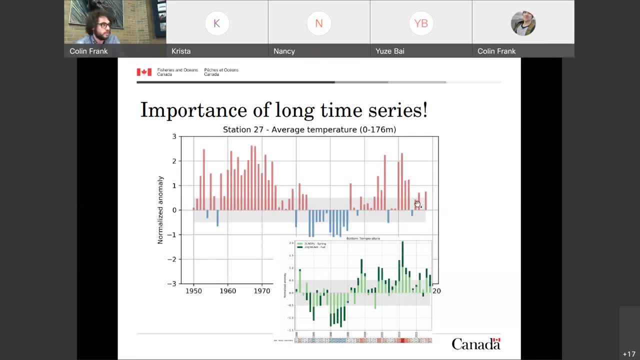 and i can least, based on 2020 and 2021, we're back towards, uh, an increase. um, how long is going to last, i'm not sure, but what you can see is that, uh, and the reason why these cycles are so slow is because they're kind of inertia in the system. this, you know, when you build this volume of cold water. 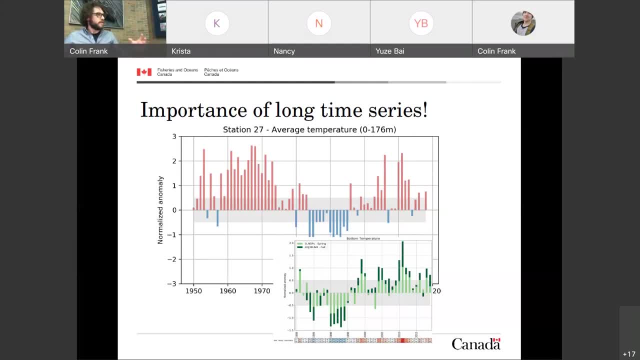 you cannot get rid of it from one year to the next. so this is why there's kind of low frequency pattern because of these, of this kind of buffering effect of how much water you have in the system versus uh, versus none. so in this aspect, yes, there is some kind of 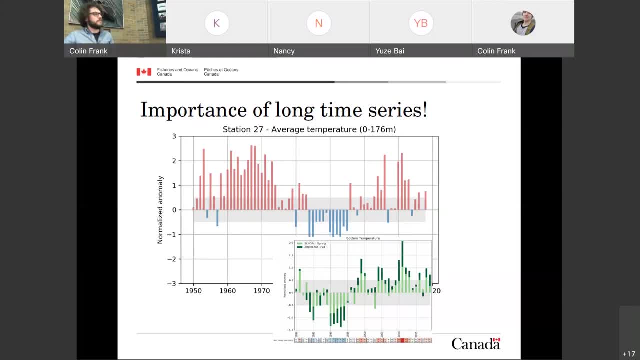 predictive power, because, uh, we know that these cycles are relatively still any more questions. i think that about wraps it up, um, yeah, so next week's talk is going to be dr andrea uh brendam uh bucheltz on marine ecosystem impacts and management responses under 21st century climate change and she.